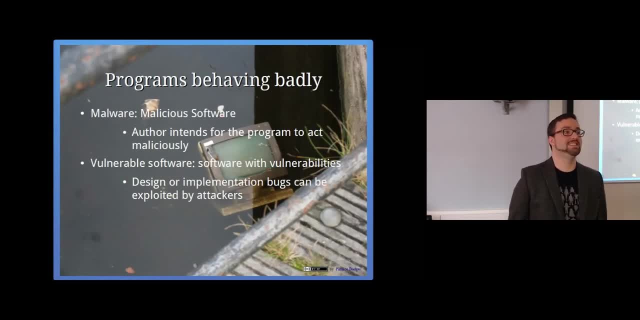 of this. There's malware, which is software that an author has intentionally created to be malicious. So the person who sat down to write the software thought, okay, I'm going to do something on this person's computer that they don't want me to be able to do. 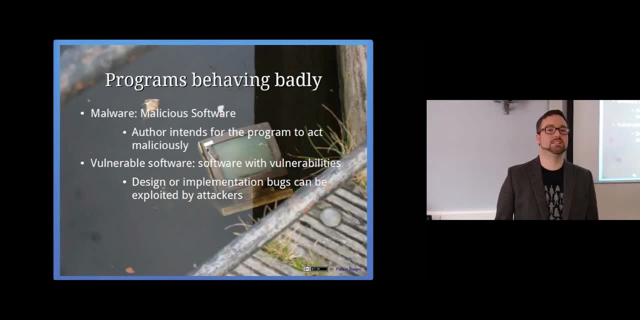 Or there's vulnerable software. so the author of the software is actually trying to do the right thing, but makes an innocent mistake, Which means that essentially, someone can attack your computer because the software that you're running is vulnerable. But both of those things are related to the same problem. 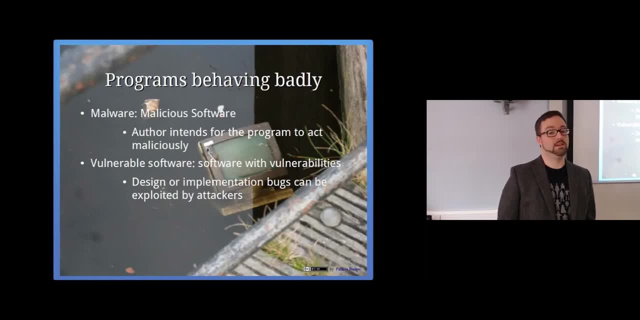 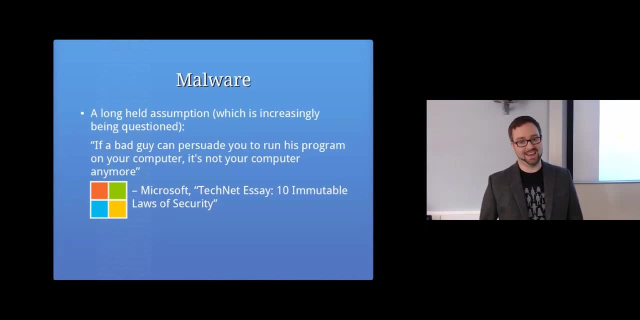 is that you're trusting the software that's running on your computer to be working in your best interest, But that's not always the case. So Microsoft even has a TechNet essay that they wrote quite a while ago now that was released. It's called Mutable Laws of Security. 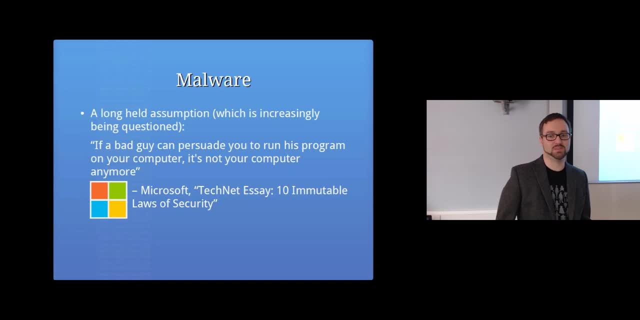 One of the best quotes from this essay is: if a bad guy can persuade you to run his program on your computer, it's not your computer anymore, So that's from Microsoft And obviously that was written a while ago And hopefully things are starting to change, where you're starting to be able to run some 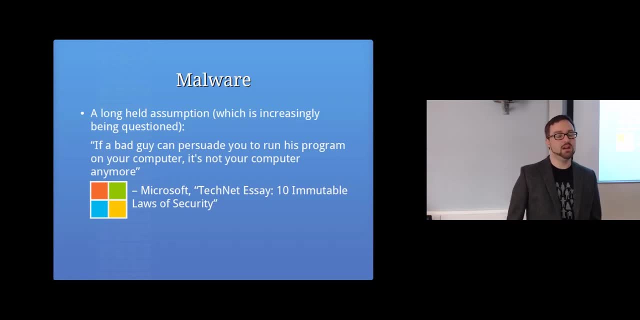 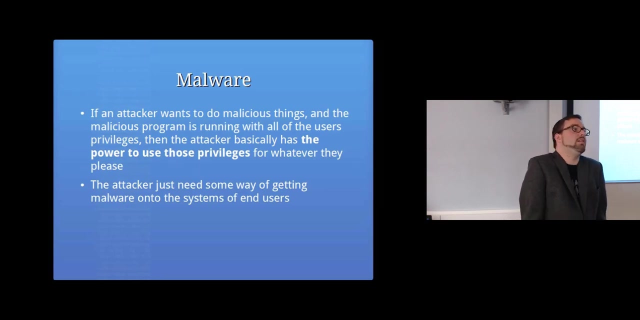 software without it doing horrendous amounts of damage. But that was the design. basically is that a program on your computer can do anything. So if that program's running it can basically use whatever permissions you've given that program to do anything that program likes. 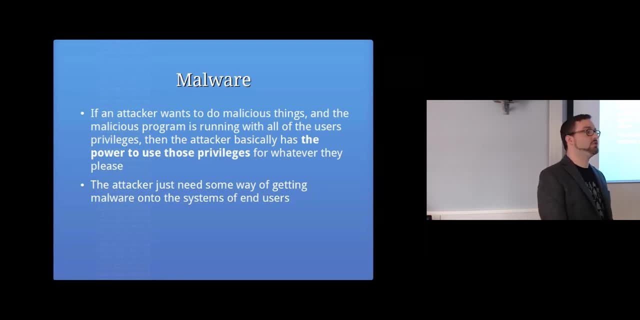 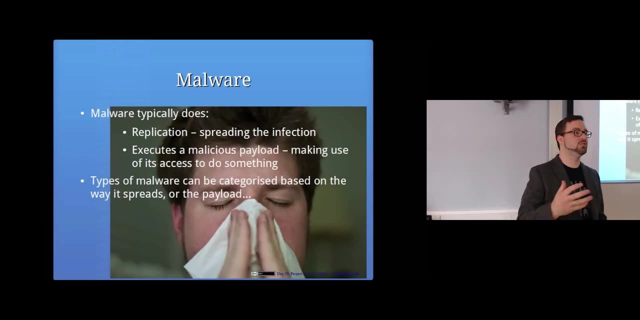 So it's just up to the attacker to find some way to get that software onto your computer. So usually what malware does is it does two things. It does replications, So it has some way of spreading the infection from one thing to another. so one device or 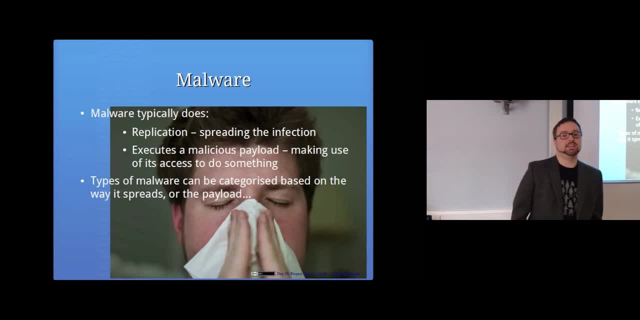 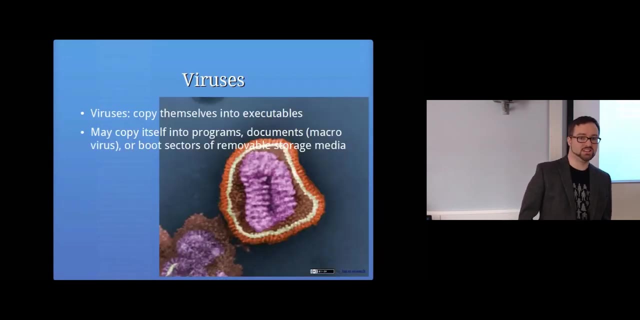 one computer to another computer And once it's there, it'll execute a malicious payload. So once it's actually found its way onto a computer, what does it do? And there's a few different ways you can categorize malware. So there are viruses, which is essentially malware that copies itself into other executables. 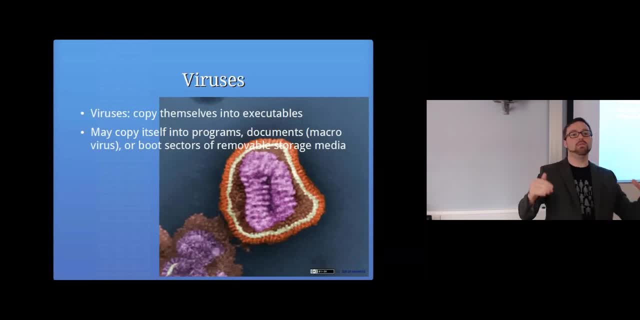 so other programs on that computer So it spreads on that same computer to other places. So it'll spread from it, might infect all of the programs that you've got on that computer with that virus. And then if you took that virus, that program that's been infected, and put it on another. 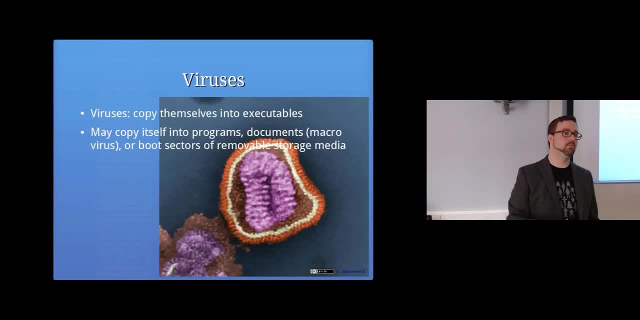 computer, then it would spread itself to all the programs on that computer. But a virus is All of it, All of it. It's also used by the media often to just mean any kind of malware. but specifically it's a kind of malware where it spreads within the computer. it's on to other programs or 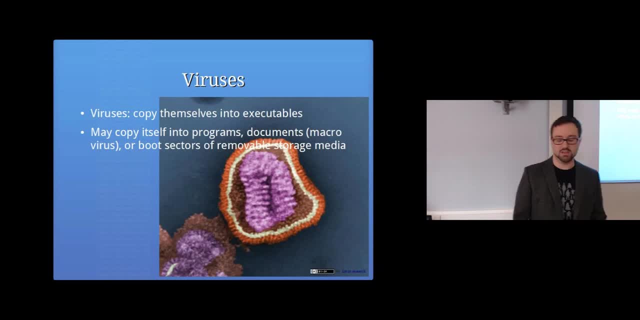 into the boot sector of storage devices. So the old way that computers would infect each other is that you plug a floppy disk into a computer that has a virus. The virus installs itself onto that floppy disk and then you carry that floppy disk to another computer and you plug it in and then you boot off that disk. 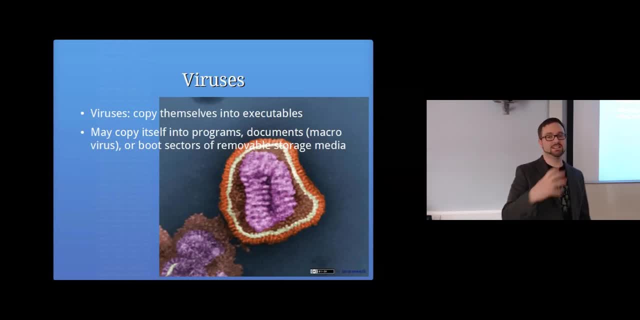 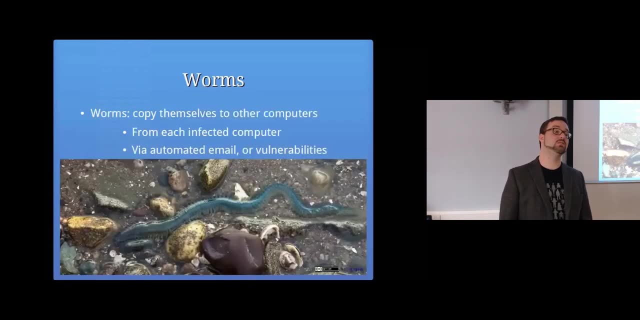 And then that computer gets infected. So it's not aware of the network. It's not doing anything to attack other computers over a network or anything, because that's what a worm is. So a worm is a piece of malware that copies itself from one computer to another computer. 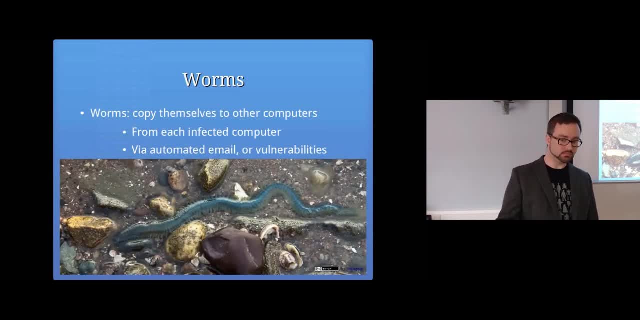 So it has some way of getting to another computer, Some ways that it might do. that is just by sending spam emails, for example. it might look at all of the emails, All of your content, All of your content, All of your contact list. 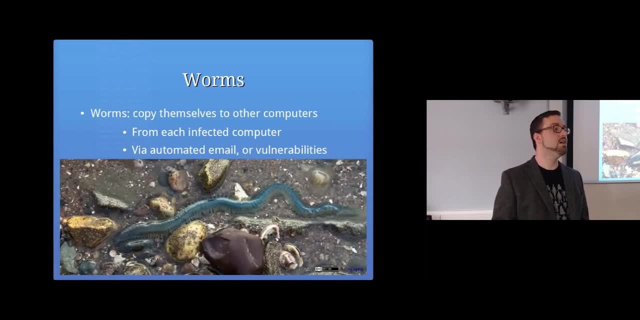 Send out an email to each person that you've contacted in the past with an attachment. That's a quite simple type of worm And then, if you managed, if the worm was clever enough at the way that it phrased it- maybe it'll trick all of your friends into opening this attachment, which then infects their computers. 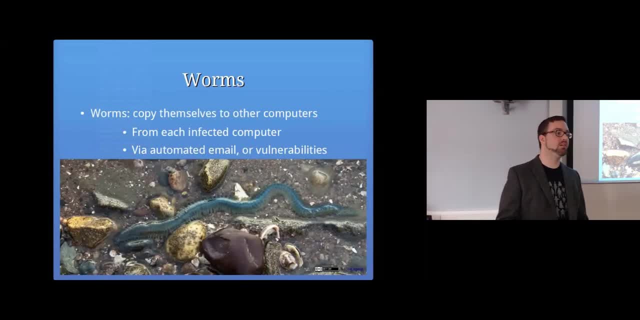 and then the same thing would happen, Or it might be more sophisticated and it might be via a software vulnerability, So the worm might actually scan the network and look for vulnerable systems on a network and basically exploit those vulnerabilities to take control of the computer based on. 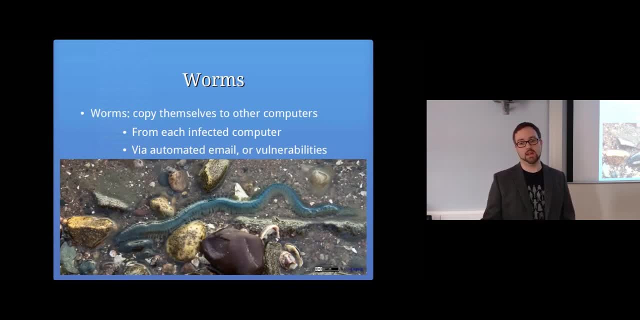 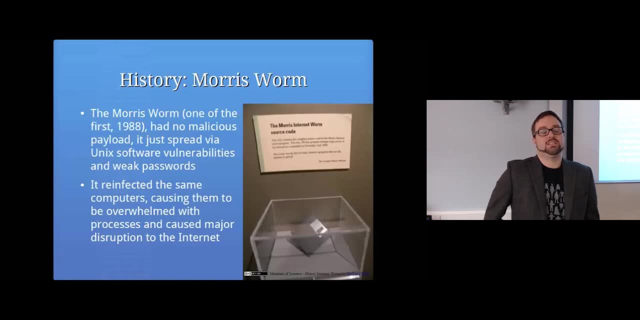 the fact there was a programming mistake there And software vulnerabilities and the details of that is something that we're going to start going into next week. So the history of malware Morris Worm was a very important thing. It was one of the first worms that had quite a big impact. So it was from 1988. There was no payload. There was no payload. Not intentionally, It just spread via software vulnerabilities and weak passwords onto other Unix systems on the network. But because of the way that it was coded it actually reinfected the same computers. 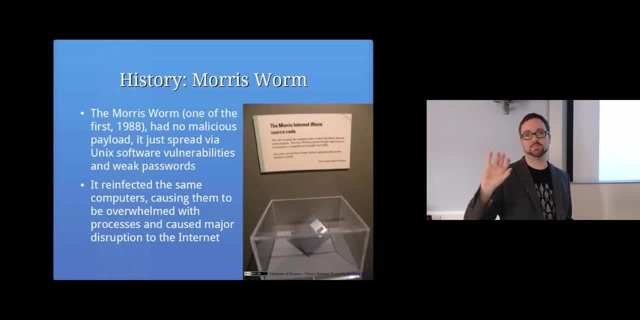 over and over again And there was some code built into it to try and limit itself from doing that. But it did spread back into the same computers and that caused computers to be basically overwhelmed. So it did cause a major disruption to the internet. 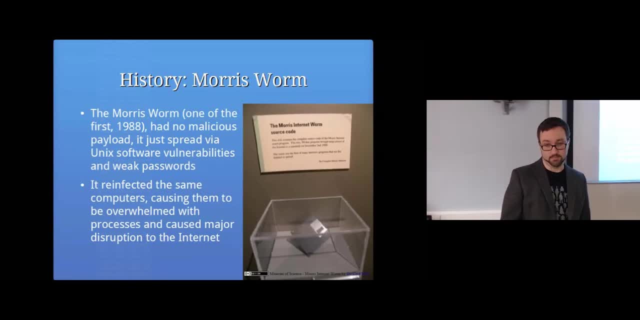 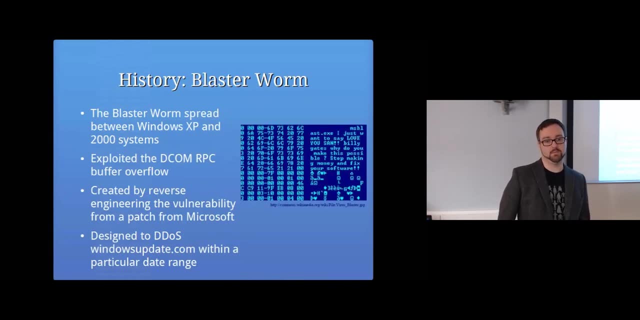 Big chunks of the internet stopped working. Blaster Worm, a little bit more recent, was another very big incident, where it, spread between mostly Windows XP and Windows 2000 systems, exploited the RPC Decom buffer overflow, which is a vulnerability that we'll look into in a bit more detail in the following weeks. 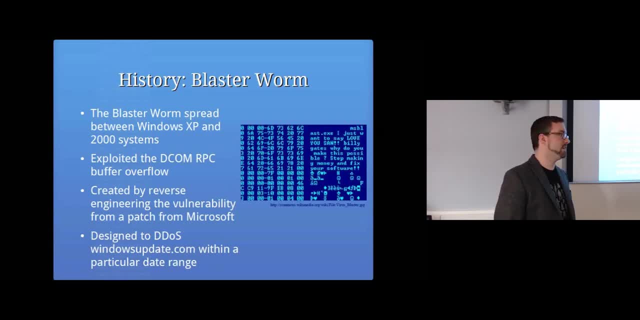 So it was a very big problem. So the way that they figured out how to attack that vulnerability is actually by reverse engineering the patches that Microsoft released to fix the problem. So Microsoft put out a Windows update. we'll fix this security problem that's been discovered. 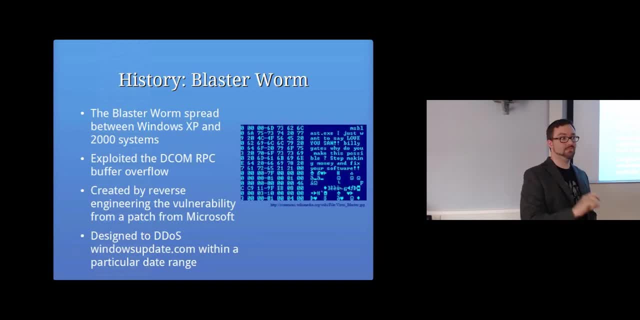 And then they looked at what changes have been made, What was the update doing, And then from that figure out how to actually attack the system And then, once all these computers that are being infected- Okay, So, once they run their payload- they basically tried to do a denial of service attack. 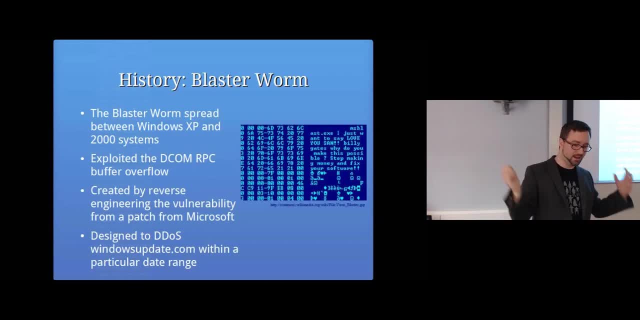 So distributed denial of service. so all these computers started trying to overwhelm WindowsUpdatecom, And it didn't work very well because WindowsUpdatecom is just an alias for another domain name. So they just switched it over and stopped the attack, But it did cause a major disruption in terms of the number of computers that were infected. 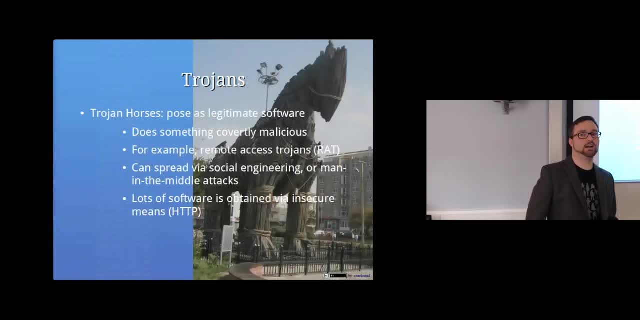 So another major category of malware are Trojan horses or Trojan. Essentially, Trojan horse is a program that looks like it does one thing but it does something else. So if you send someone that you know a game and say, hey, run this game. 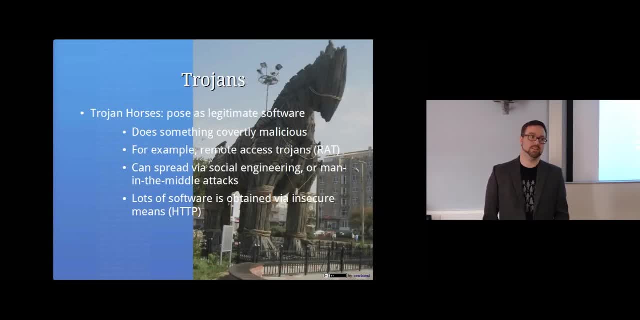 And it actually does something else to their computer and that's a Trojan horse. So it's got a covert and an overt action. So the overt thing- The thing that it does, that the person is aware of, is benign, and the covert thing is: 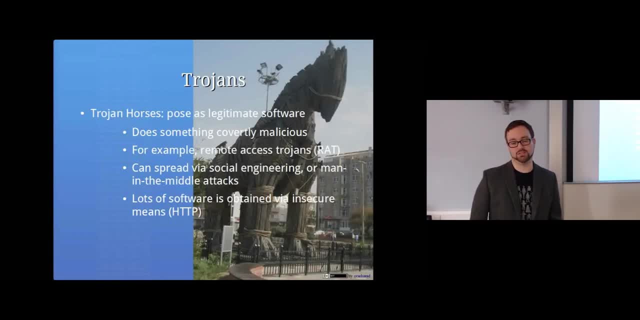 malicious, So it's doing something with that person's resources that they don't want it to do. And one type of Trojan horse is a remote access Trojan or a rat, which is essentially a Trojan horse that gives someone else the ability to log in to their computer and basically 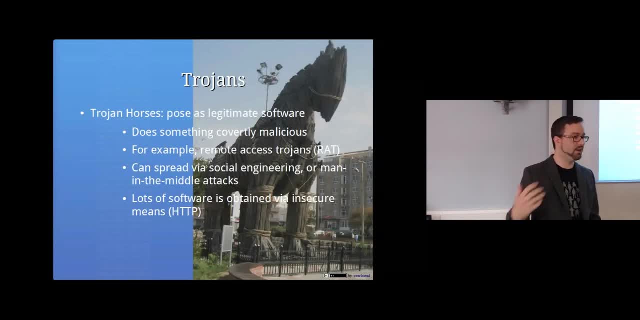 take control of it And they might have access to all the files on that computer. they might be able to upload files and download files from that computer- A lot of them. you can move the mouse around and do annoying things like that, which I. 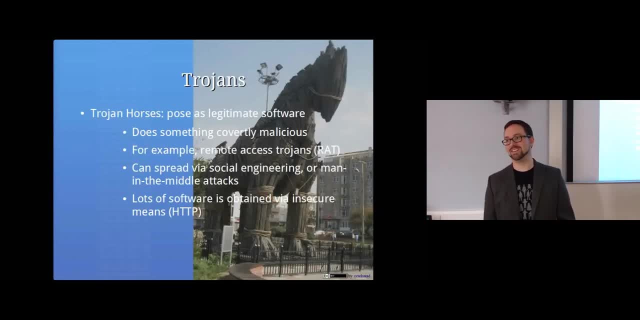 think you guys have experimented with. Last semester we did a little introductory session, which was quite fun, but obviously the realistic things that can go wrong can be quite severe in terms of black businesses And if you get access to confidentiality, Yeah. 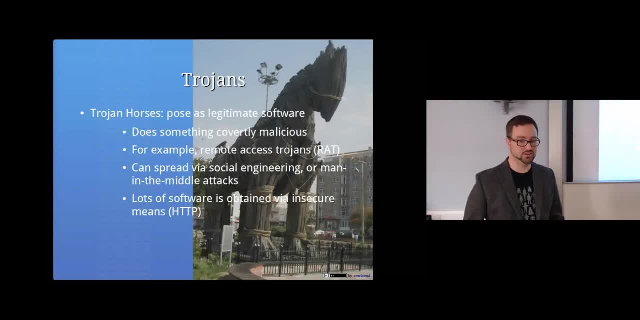 You can get access to confidential information. So how do you get a Trojan horse onto someone else's computer? Often it involves some kind of social engineering, So tricking that person into thinking it's okay to run the program or that that program is going to do something for them. 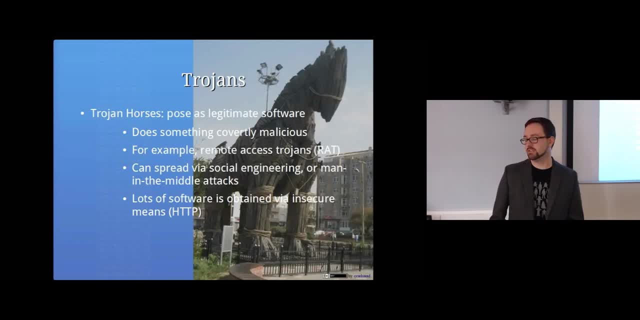 And that might be in person or, more likely, just via digital means, like an email or a USB left lying around, And there's also man in the middle attacks. So you might actually be connecting to a website that you do trust, but then someone might be interfering with the network connection and actually substituting out the software. 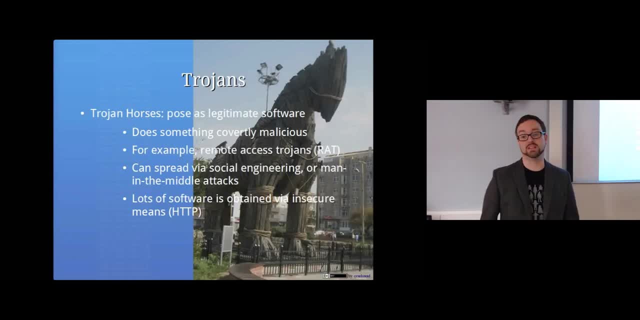 that you think you're accessing from a secure place and you're actually downloading it from the attacker. There's all kinds of different ways that you can end up with malware instead of what you're expecting If you download software via torrents and stuff. it's something that you should definitely 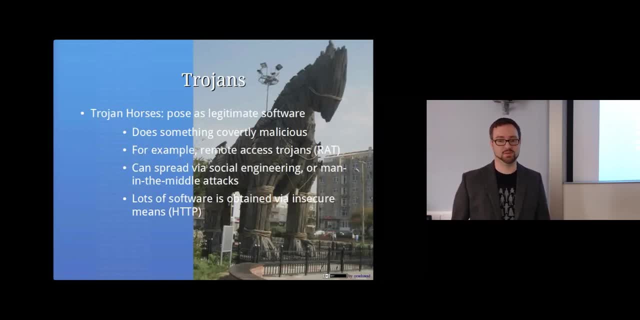 be concerned about. It's like: how much do you trust them? Yeah, There's a lot of people that put that software on there to actually be the software it says it is. So we actually do obtain quite a lot of software via insecure means. 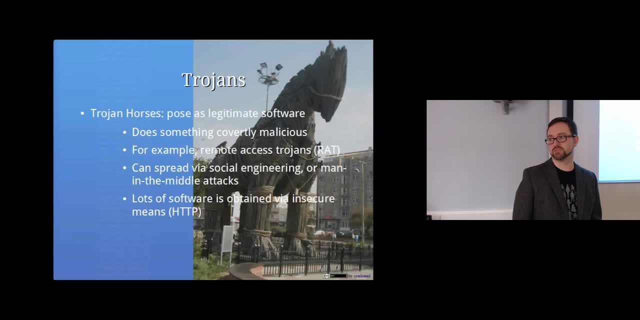 So if you're ever on a website that's not doesn't have any encryption, for example, so if it's just HTTP traffic, then there's very little security in terms of making sure that you are actually accessing the website that you think you're accessing. 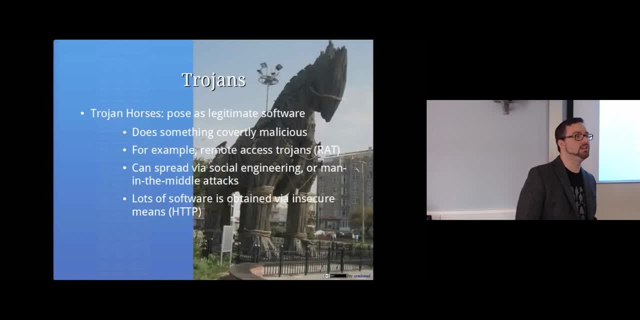 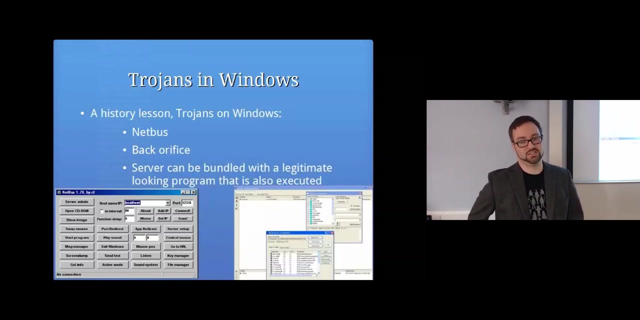 So if you're downloading software from a website where you are not sure, not 100% convinced, that that software is actually as intended by the author and from a secure location, then yeah, then you've got reason to be concerned. So some of the historically important Trojan horses in Windows were like in the 90s there. was like Netbus and Bacorifice, Yeah Yeah, And a whole slew, a whole bunch of Trojan horses came out around that time And at that time Windows didn't really have. it was a simpler time that Windows often didn't. 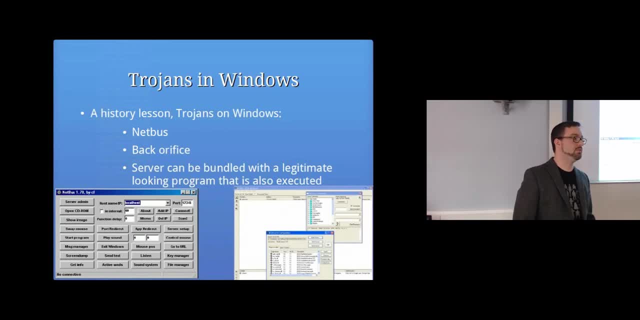 have a firewall at all, So there's nothing stopping someone from connecting into the computer once the Trojan was running. Everyone had a publicly accessible IP address because you know it was before we used network address translation for like every router in someone's home. 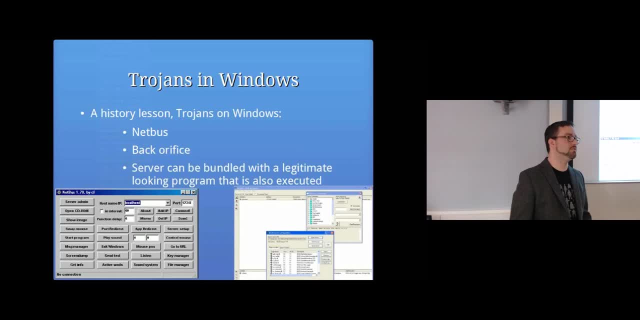 So you could literally just connect in to someone's IP address or scan an ISP for ports that are open for people that have been infected by a particular Trojan and just connect and start controlling their computer. It's still. it's still definitely possible. now it's just slightly more complicated. 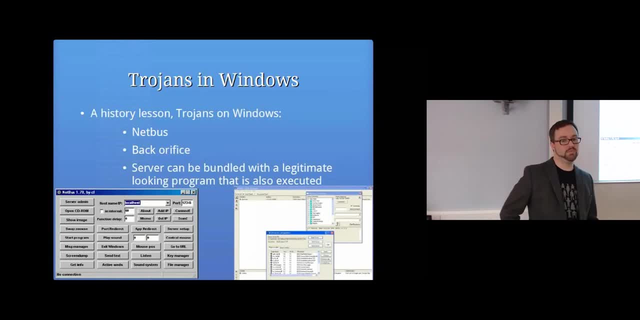 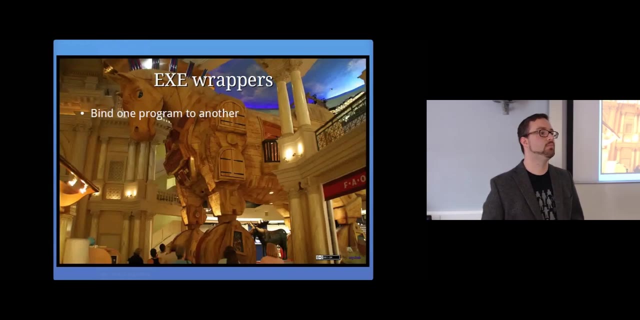 So those are just slight technical barriers, but definitely it's still just as big of a problem, basically, as you'll discover in the lab exercises from this week. So an exe wrapper is basically when you take two programs and bind them together so that 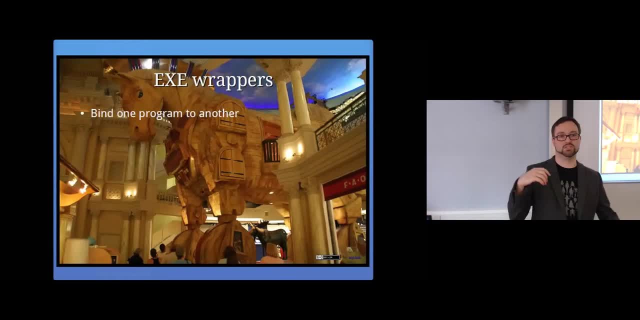 you create one exe file, you run it and it actually runs both of the programs that you then that you had put together to create this. So, for example, you could take a whack-a-mole game and combine it with Netbus Trojan horse. 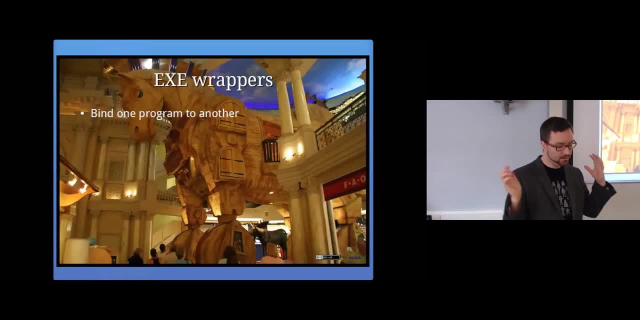 so you know the server component of that- generate a new executable and send it to someone And then when they run that program, the game really does start. So for all they know, oh, you did send me a game and it looks like an actual game, but 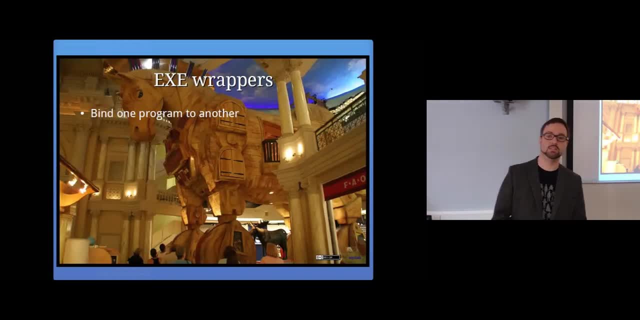 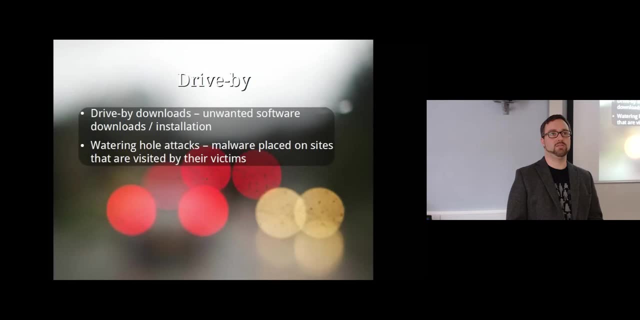 the server's also running and your computer's been infected by Trojan horse. So drive by downloads is also another problem. So you know, often when you're browsing on the internet you know there are certain pages where you'll, you'll, you'll go there. 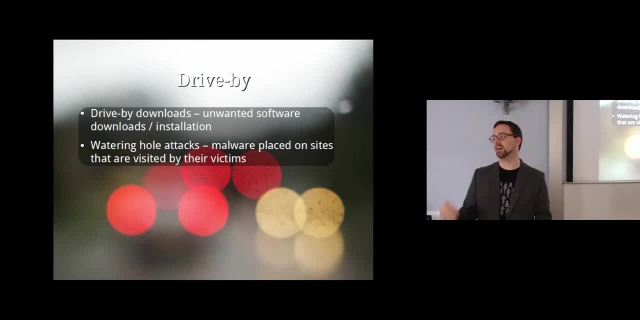 And it will just pop up and prompt you to like download an executable file or something, And if you don't understand what that means, you might go. oh yes, this is just part of me accessing this website And you run the program. and well, you've just lost as soon as you've run that program. 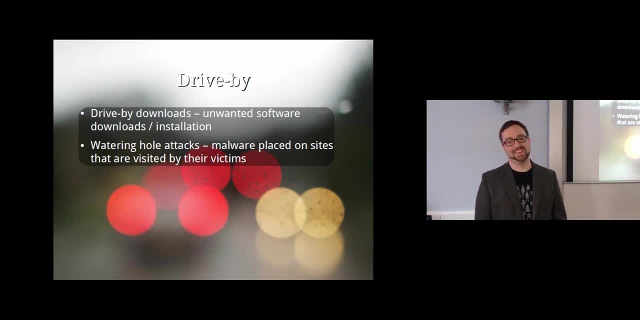 as Microsoft have just explained to us, The watering hole attacks is where you basically create or break into a website that someone is likely to want to access And put malware there. So, for example, there was an attack that was discovered against Apple employees, the software. 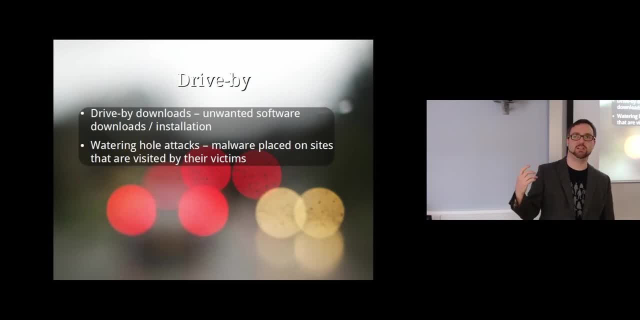 developers where they. this is a few years ago. they had some developer website that they used to access a lot and that actual website had been compromised. So some of the tools that were available there were actually, you know, Trojanized software. So yeah, 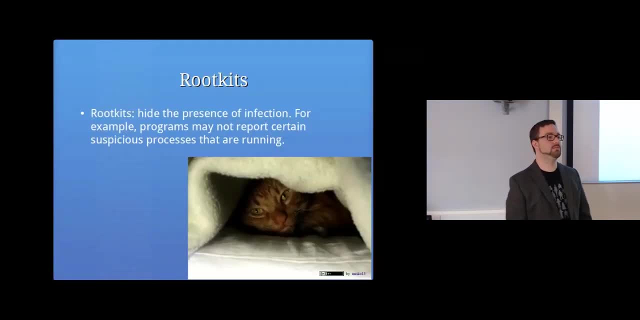 So Rootkit, How many of you guys have heard of the Sony Rootkit Show of hands? Jesus, It wasn't that long ago, guys. So, yeah, it's amazing. So it was okay, so it was, it must be a decade ago now, actually. 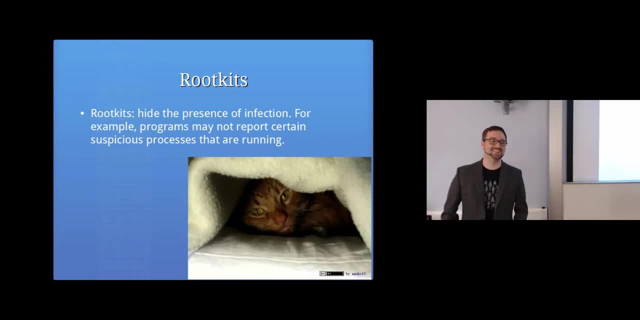 So it was like Beastie Boys era. So Sony got into quite a lot of political Pressure for basically bundling a Rootkit with the albums that they released. So you know, digital rights management is software that's designed to stop people from copying music and all that sort of stuff. 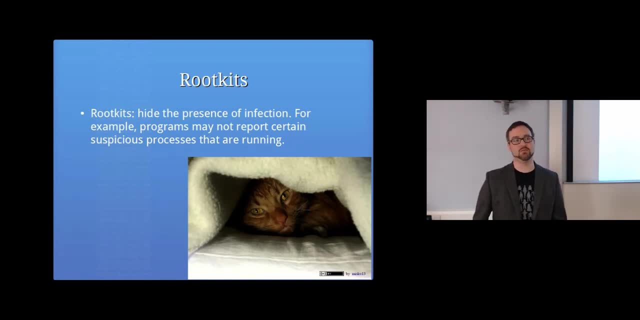 So their solution was, I know, let's infect all of their computers with everyone running Windows, which most people at the time in the 90s- was it the 90s, 2000s, 2000s, I think? 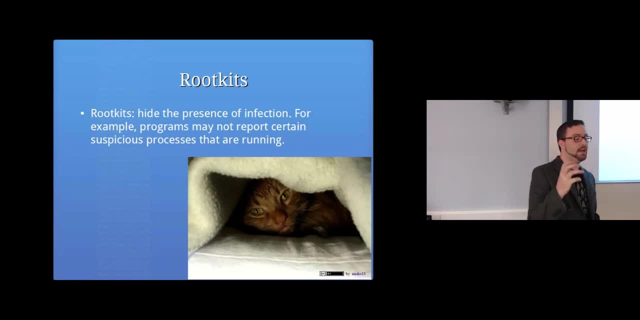 So they basically Yeah, Yeah. So if you got like the latest Beastie Boys album or a bunch of albums that came out of Sony at that time and you put it in your computer and you close the CD back then, so it was Windows was automatic, default was to run whatever software was in the disc that you put into. 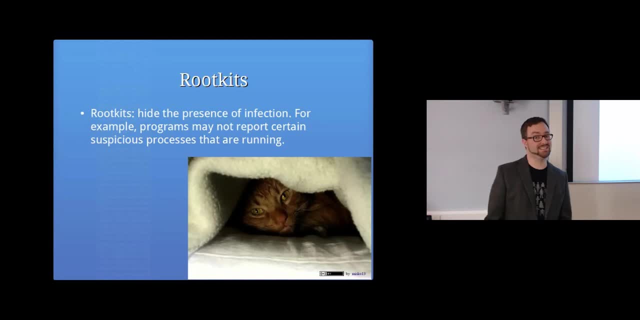 the computer. For obvious reasons, that's not always the case anymore, but sometimes still is. So you'd put the CD in and would install the Rootkit, which is basically a Rootkit is malware that hides itself from the audience, From the operating system and from the users. 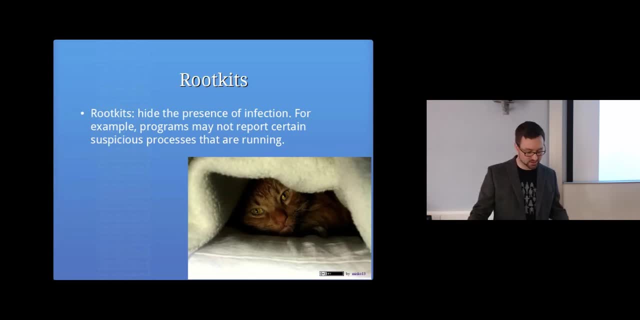 So that if you go looking for it you can't see it's there. So you know, on Windows you press like Control Shift Escape and it comes up with a list of processes. It won't show the Rootkit in there because it's like hiding it. 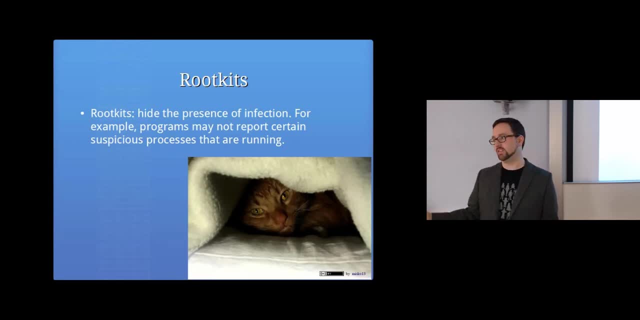 And if you go and look through the file directory and stuff, you won't see it, the stuff that's there, because the Rootkit is hiding it. So essentially it was hiding itself so that it could try and stop you from copying music or whatever. 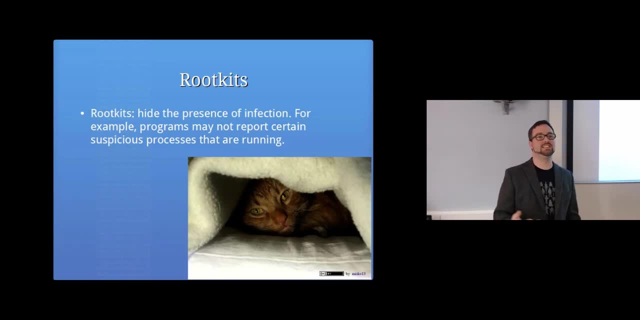 But also as a. consequently, it made it easier for Other malware or other attackers to basically hide stuff on your computer. because it was just it did something like: if your file is named a certain way, it just hides it. So other malicious actors basically took advantage of that and started using the Sony Rootkit. 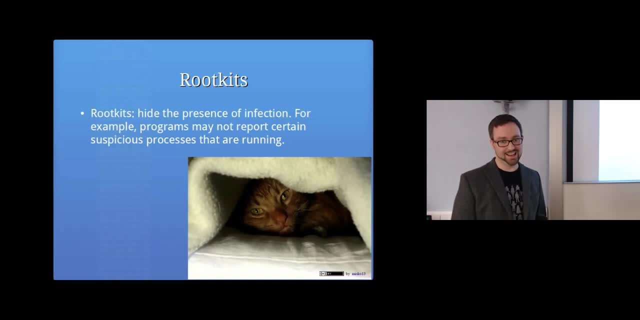 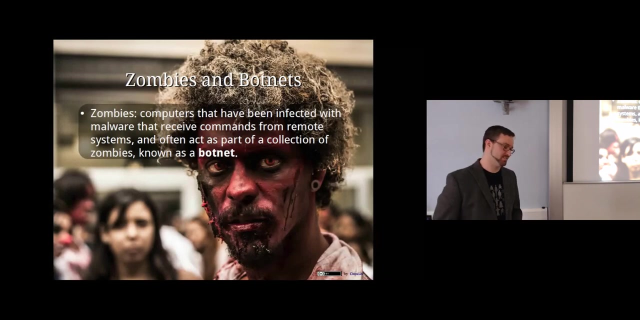 to hide their activities on computers. So, as you can imagine, it didn't go over very well, But then again, if everyone's forgotten about it by now, then they should be quite happy about that. Zombies and botnets. So a zombie is basically a computer that's controlled by someone else. 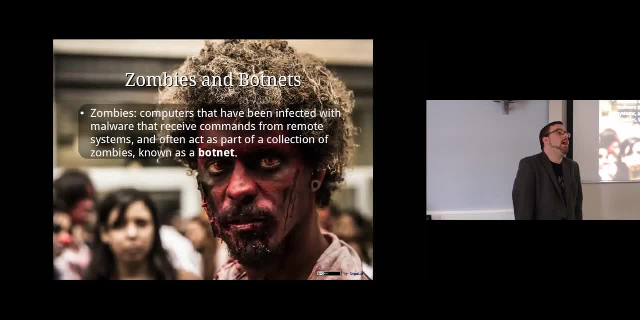 So it's a computer that's been infected and now is essentially, whether you know it or not, is owned by someone else. So they have the ability to make your computer do stuff, And so they'll send or they'll receive commands from remote systems. 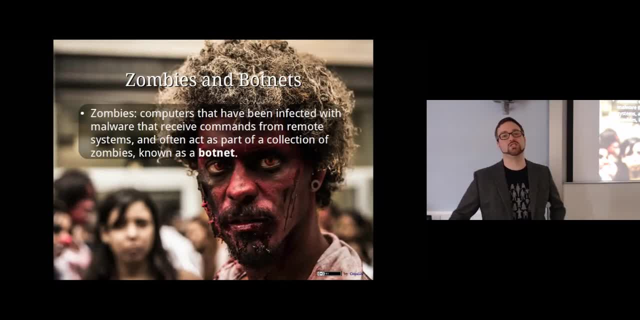 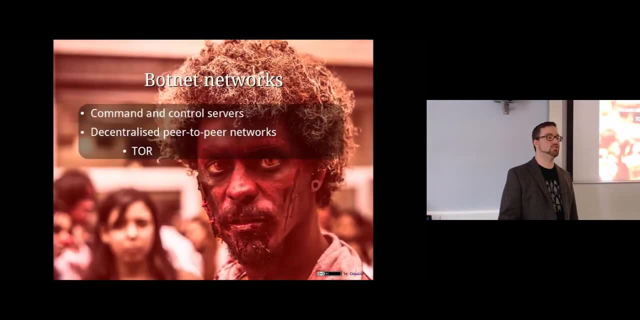 And a collection of zombies is known as a botnet, So a collection of computers that are all being infected and that someone controls. And the traditional way that it worked is you'd have command and control servers, So you'd have a central server that all the other, all the zombies connected to. 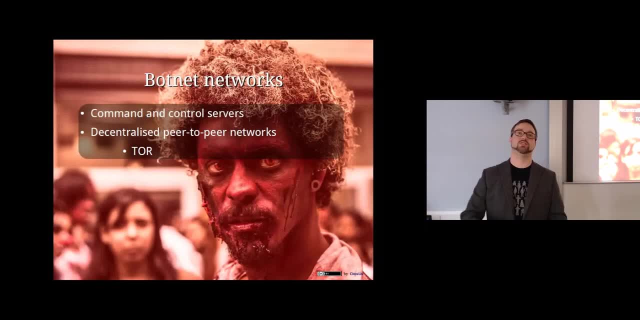 And then the botnet controller or the master of the botnet or whatever, would connect into that central server and then be able to issue commands to the others. Nowadays they're getting more sophisticated and they're distributed, So it's more like a peer-to-peer network where they, the zombies, associate with the swarm. 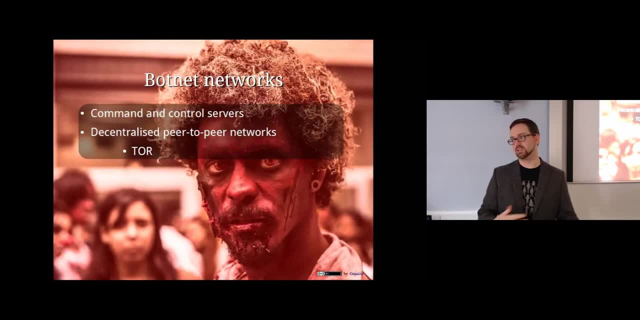 of other zombies and they can share the information and the commands with each other, So that you know, the person who's in control of the botnet can just connect into any part any one of those systems and issue a command that then just get filtered through to the. 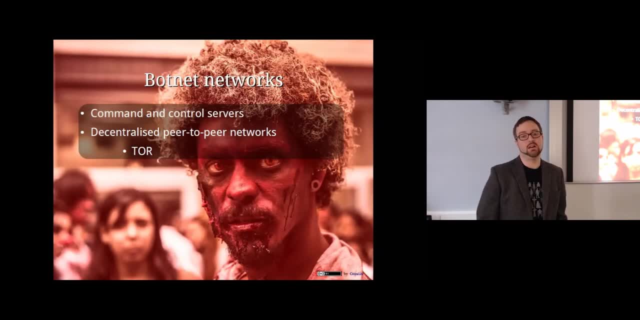 rest of the to the zombies on the botnet And you also have you know They might start using Tor and other ways of becoming more anonymous. Yeah, So it's not like the um the botnet does all the anonymous trying to or to do this. 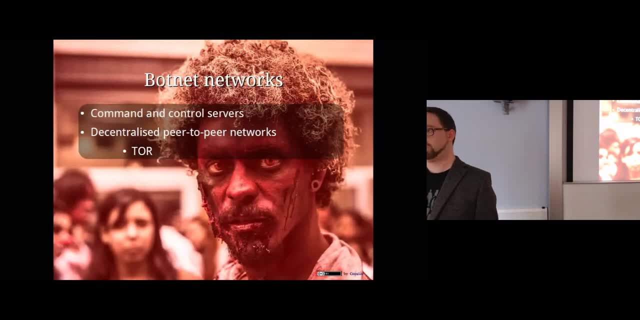 everything to the immunity called IO-Connect Yeah, Which is essentially um, we get to an IRC server or a hive, everyone's getting to that, and then somebody's sending commands from the hive and everybody, the botnet might deploy it from something else. 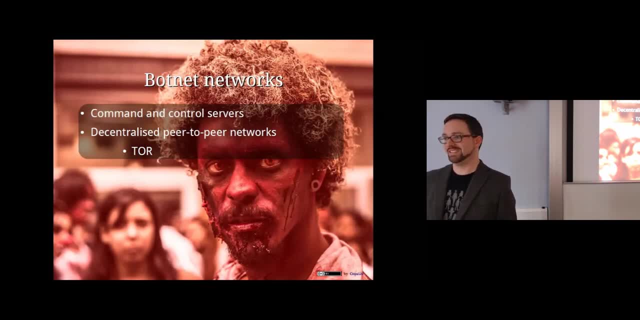 Yeah, That's like being a willing participant of a botnet. Yeah, So it's so, yeah, So, yeah, it's a good point. So that, yeah, So anonymous. So just to repeat: Uh, partly cause this microphone's not good for catching what you're saying, but yeah. 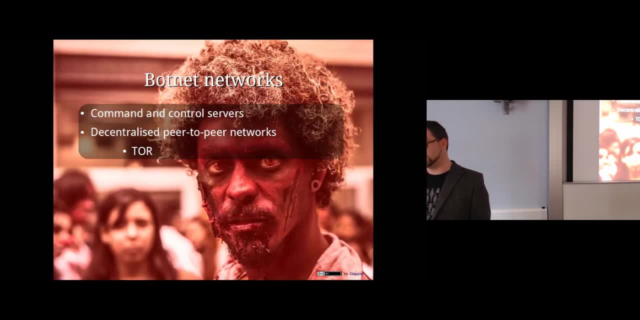 So it's a good point about the software that um, the anonymous used, where people can basically opt in to be, have these commands sent to them and then their computer would then start attacking um, you know, whichever computer that the, the hive mind of anonymous, decided. 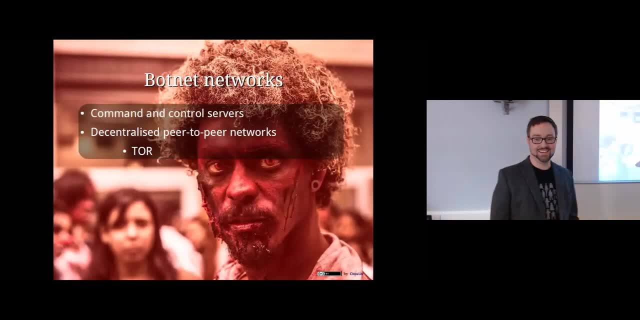 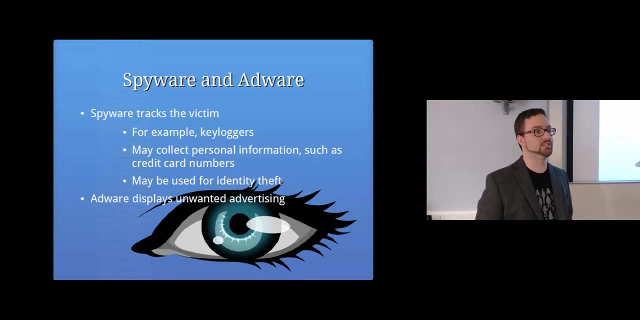 to attack. Um, yeah, Um, spyware and adware. So, um, spyware is basically software. Yeah, So there is basically software that tracks the victim. So, for example, a key logger. say, um, if I install a key logger on on a computer and 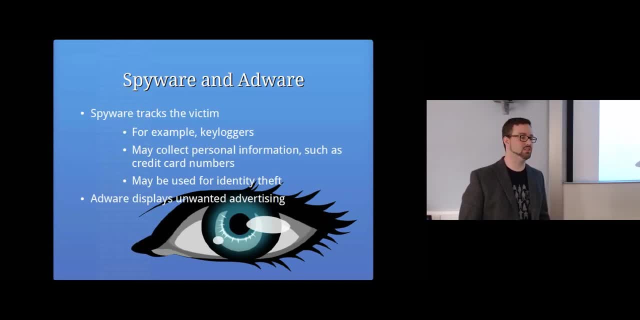 someone else walks up to it and starts typing stuff in. So, for example, they log into, um, their bank account or um, you know, PayPal or my Beckett or whatever. then, um that all of the things that they typed in is logs to a file. 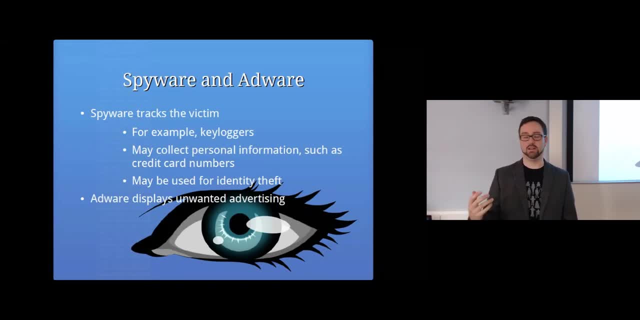 And I go back up to that computer and grab that, that, and then I've got access. I've got access to everything that got typed on that computer. So it's quite a serious like from a privacy point of view can be quite, um, quite a serious. 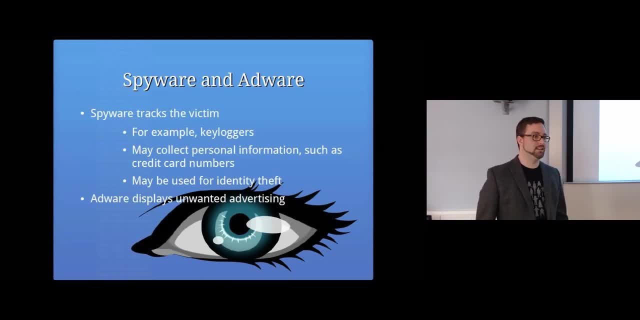 problem. So the sorts of information that can be collected is obviously passwords, but also credit card numbers, Um and um. if. if you collect enough information, obviously it you may be identity theft. So if you manage to, you know, get access to someone's email account, um, that obviously. 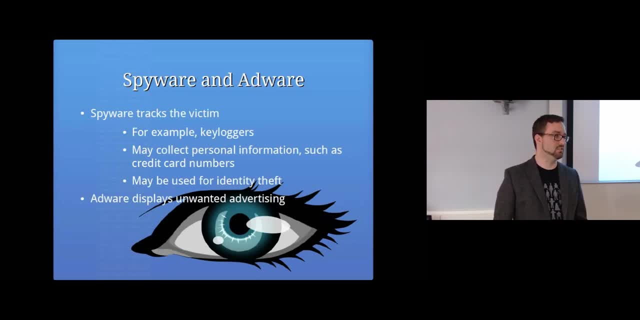 um, you know, um That often gives you access to basically everything else because click, I got my password on whatever website. it is, Um, yeah, serious problem. and and adware is malware that displays unwanted advertising. So, and where you draw the line between um adware and just annoying ad based revenue? 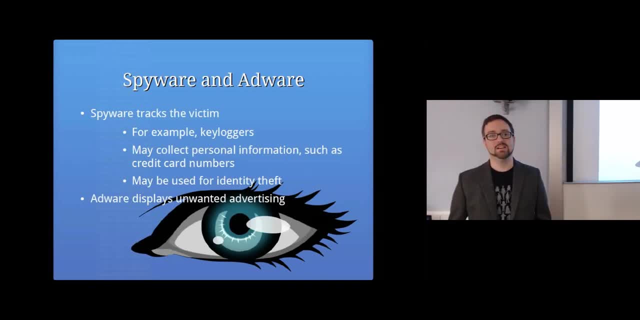 driven programs, um, is, I guess, uh, kind of a bit of a blurry line. So So, basically, adware, often it's software where you're you install, I don't know. I think line wire is an example back in the day where it was like a peer to peer network. 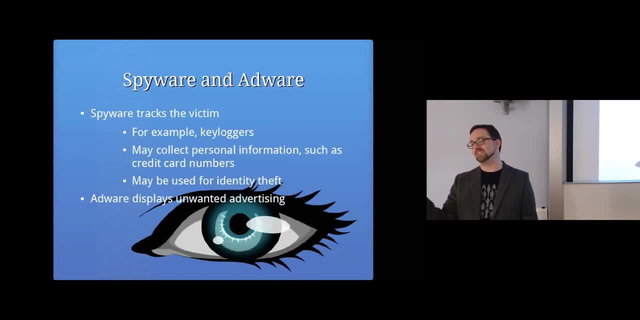 Yeah, So you download. you download one of those programs and you know you. it will actually ask: tell you as part of the license agreement that you're agreeing to it. So it's like you can't turn around and sue them, but essentially you're giving them permission. 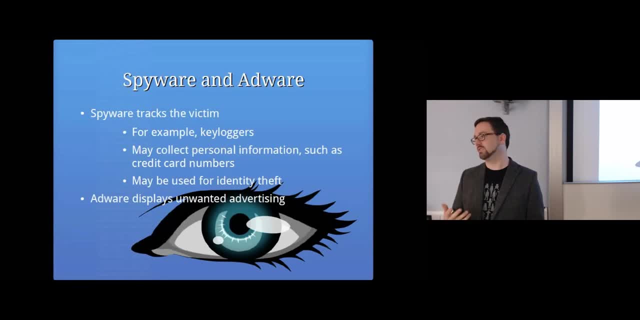 to install software that um pops up advertising on your computer, And one way it might do it would be just to pop something up into the middle of your screen, click this and you know you get all the big popups and everything popping up. but it might. 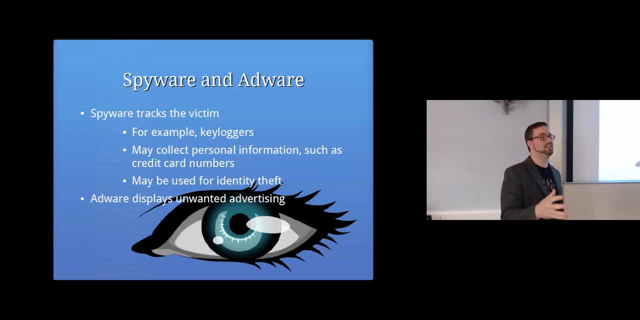 be a little bit more subtle than that. It might actually just subtly change the websites that you're already accessing to just include an extra advert or to swap out a Google advert for their advert, because obviously that you know they make money each time someone clicks on it. 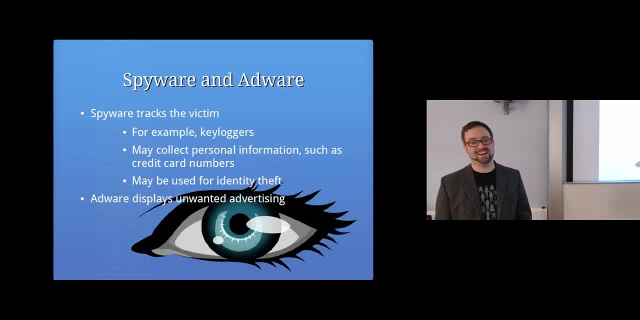 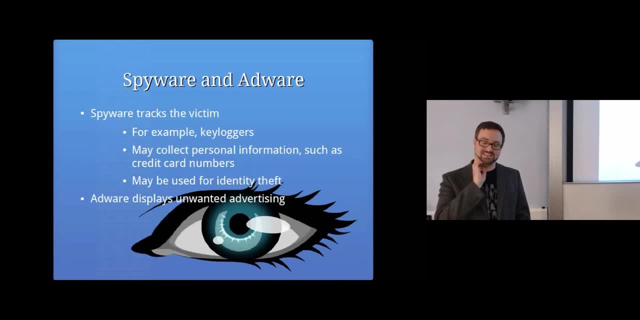 the current thing that's in the news this week is the new version of windows. So the windows 10 technical preview includes a key logger, apparently. Um, and you're agreeing to that. when you put windows 10 on your computer, you're saying: 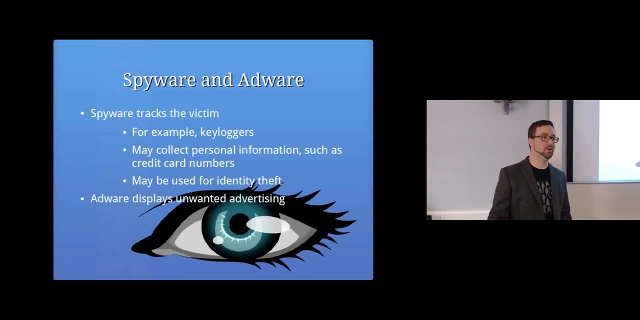 yes, I agree that everything that I type and everything I access will be sent to Microsoft. Um, It's nice, the NSA being more transparent. Um, you'd be surprised. It's not always the NSA, because the companies have quite a bit of a lot of incentive to. 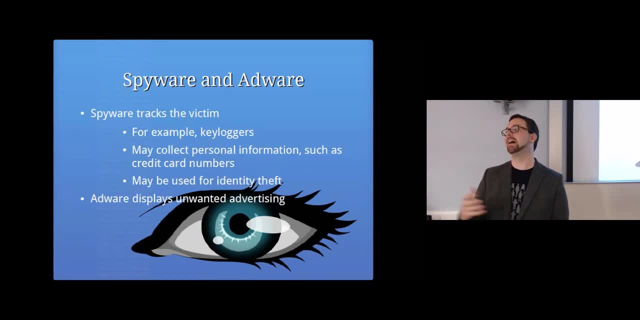 spy on you as well, because if a company knows more about you, they're more likely to successfully advertise to you and they're more likely to give you an advert that you're likely to click on. So it's not necessarily because they want to know everything about your personal life. 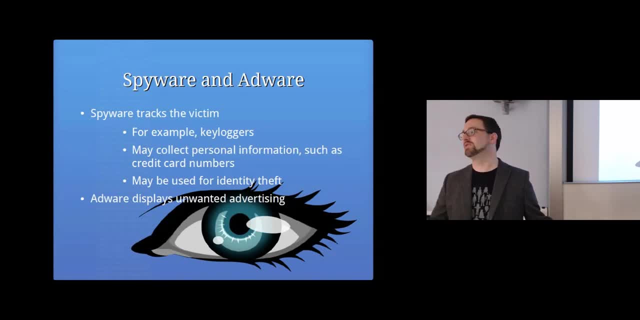 but it's because they want to make sure they can target advertising and, as a consequence, the NSA can conveniently access all that information. if they ask Microsoft allegedly, What's the difference between AdWare and the websites that remember the tree of search history and the products of the search history on YouTube? 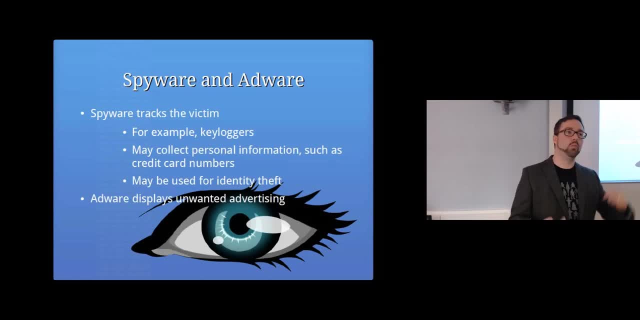 So yeah, like I said, it's a bit of a blurry line, but when cookies were first introduced it was kind of controversial and people would turn off cookies in their web browsers because it allows websites to track you. So if you're, If you don't know, a cookie is essentially when you access a website it'll generate. 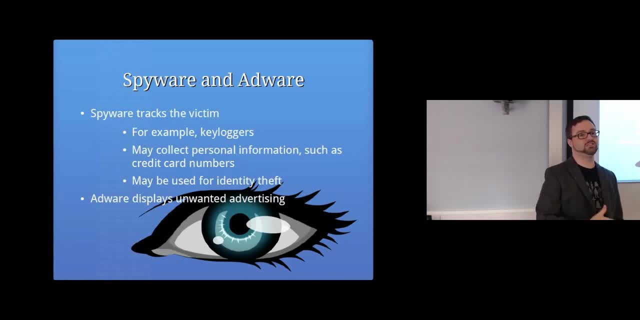 like a string or random string that identifies you so that next time you visit that website it sends the cookie through with that random thing or with your username or whatever. so then they can see it's you each time, So they can tell when you go back to the website. but if you disable cookies, most of the websites 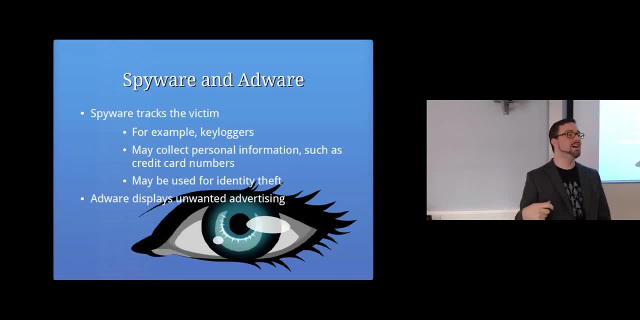 nowadays will stop working properly because they rely on that to work properly. But then you have third party cookies, which is the biggest privacy concern, which is where it's not just the website that you're logging into. So you log into YouTube or whatever and you send them a cookie, but you might also have 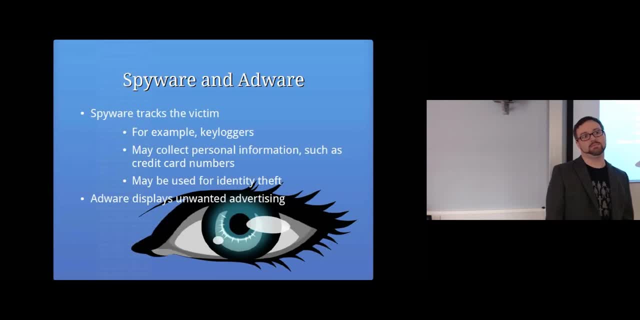 embedded in that website some advertising domains and you send them your cookie, So then they can start tracking you across all the different websites that you visit, so they can see that you've accessed this website. So, for example, Facebookcom, Facebook- the like button. 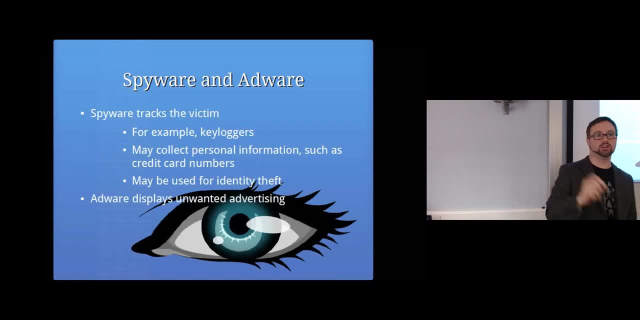 So Facebook know whenever you're at everything. So if you're logged into Facebook, they know every website that you've visited. that includes like a Facebook like button, because it sends a cookie back to them each time you access those things. Yeah, Does it matter. 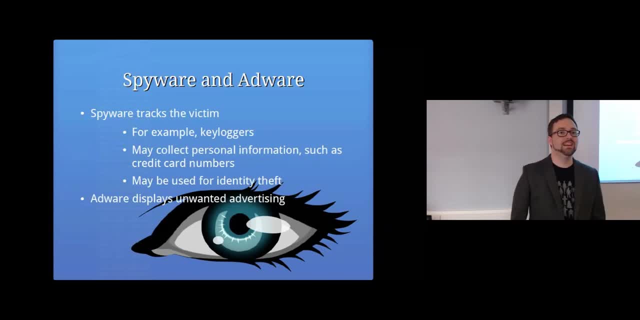 Does it actually matter that someone is tracking what you're doing? Does it matter? Does it actually matter that you're actually tracking someone that I'm never going to meet because you're reading my email? I'll do a whole. I'll do a whole lecture on privacy towards the end of the semester, but just a show of. 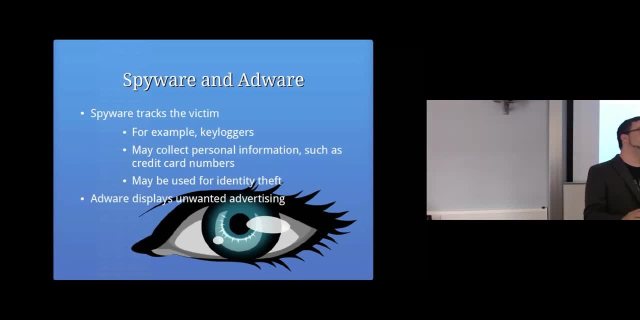 hands. A show of hands. Does it matter? Do you care? Do you mind if someone tracks everything that you do on your computer and on the internet? A show of hands. if you do mind, Yeah, And so that's the majority of people, and we'll talk about that in a few weeks. 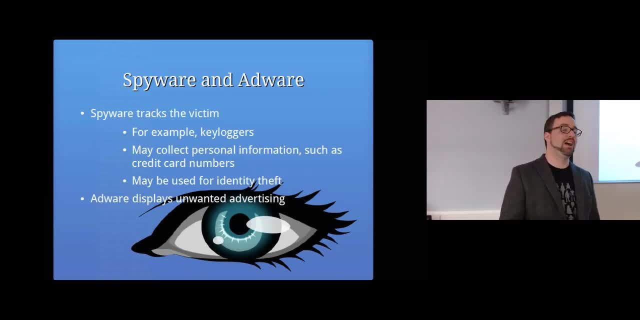 And it's. You know, maybe you don't, I'll just I'll say, I'll say one One thing. One thing about that is there is an argument that if you've got nothing to hide, then don't You've got nothing to be worried about. 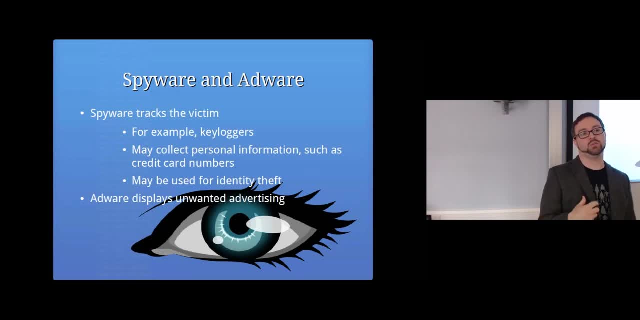 But think of the way that things can be used out of context. Think of the way that people can be manipulated and taken advantage of if you know a lot about them. That's all I'll say, But we'll talk more about that in a few weeks' time. 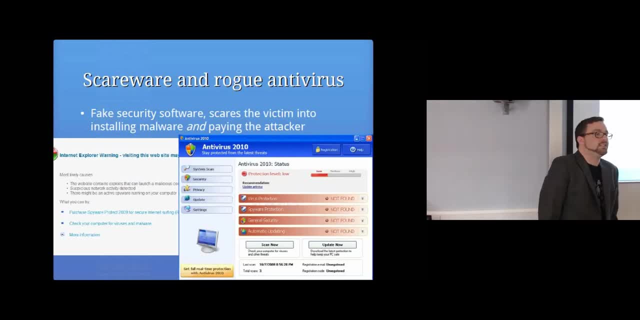 Um, So scareware and rogue antivirus is quite a common type of malware where essentially they try and scare the victim into installing something. So you might actually be on a website and it pops up and says: detected your computer's infected. Click here to fix it. 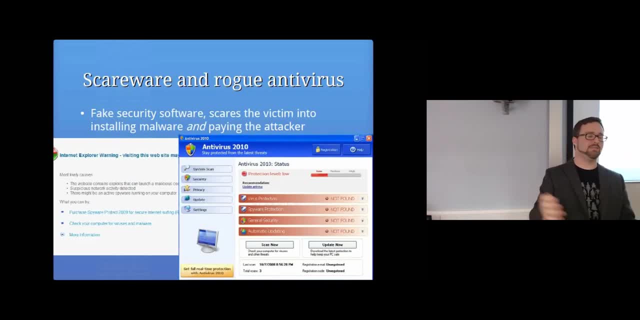 And if you're not that bright you might think: oh, the website knows about my problems and can fix it for me. You click the button and you install the software and then now you've actually got malware on your computer And it'll actually look like antivirus software itself and it'll come up and say: scanning. 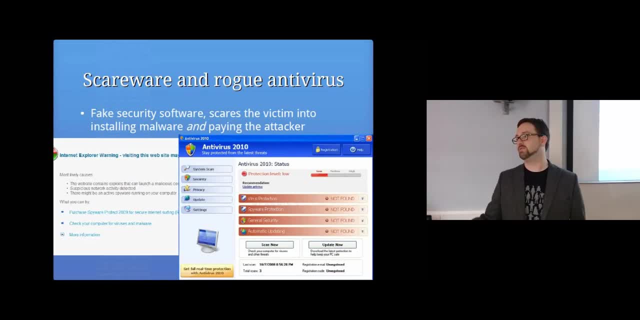 diggity, diggity, diggity. Oh, one billion- you know- pieces of malware on there. Fix, click, fix, And then do, do, do, do. Oh, I can fix half of them for you for free, But if you want the other half fixed, then pay us money. 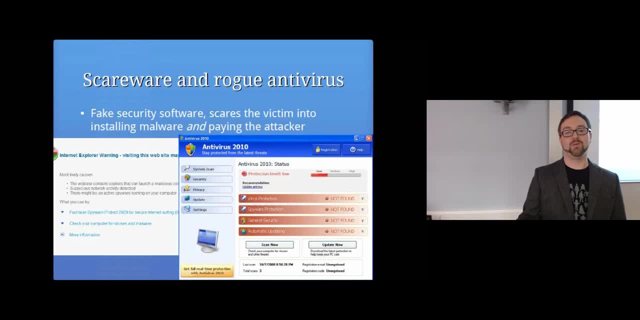 And then people actually get fooled into paying them for infecting your computer. So not only have they got malware on your computer, but they've tricked you into paying them for creating the malware that you've installed on your computer. Could it use? 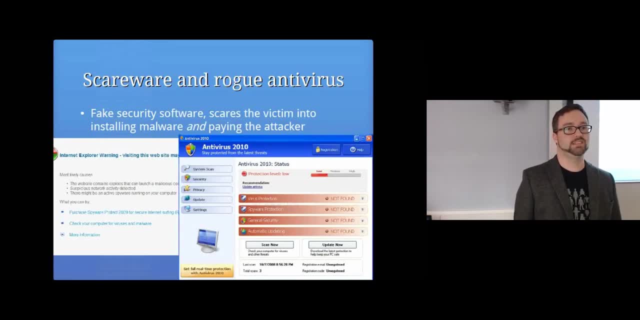 Could it use other malware to find out what antivirus software you use And then, when it produces something that looks a lot like antivirus, it could look identical to Avast or whatever. Yeah Well, actually I haven't heard of that happening, but I guess there's no reason that it couldn't. 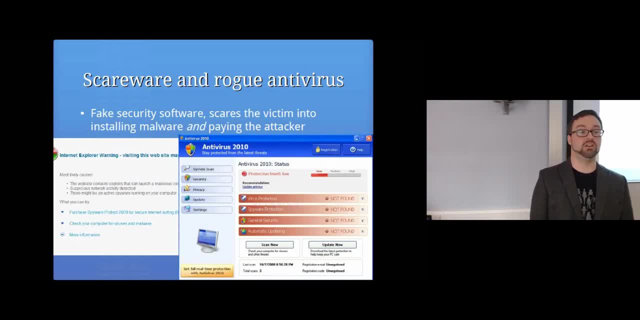 try and disguise itself as the antivirus that you've already got on your software, on your computer. You could be a good evil genius, But no, it's a good point. It's a good point. Often they will disable other antivirus software. 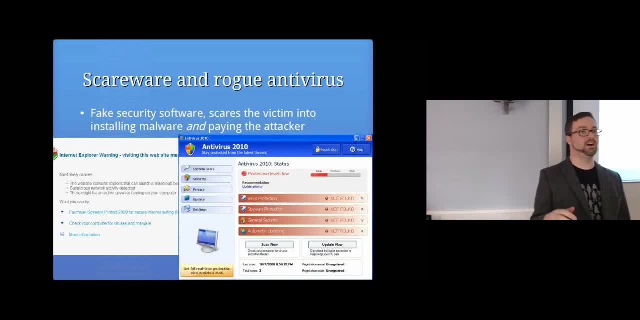 so a lot of viruses try to turn off any virus scanners. so the first thing it does is will actually disable whatever antivirus you've got and, depending on whether that antivirus software has some kind of protection against that, often you know the the malware will just turn off your anti-malware. yeah, good fun. 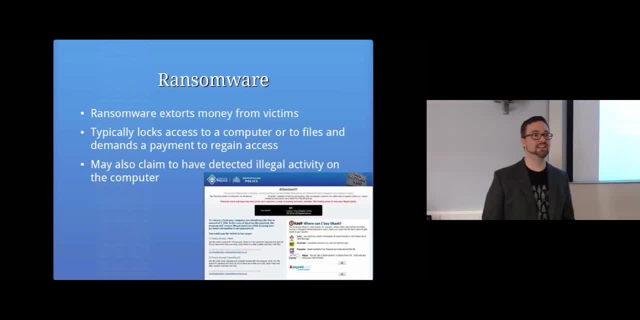 ransomware- this is like quite current and happening at the moment- is quite popular. so I'll talk just in a minute. I'll ask you whether or not you know anyone that this has happened to recently. so, basically, what ransomware does is it tries to extort money from the user, from their victims. so there's a 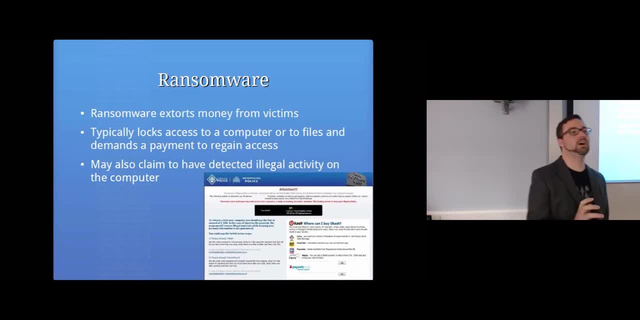 few ways that it does this, often by just locking the computer so it'll set up, it'll install stuff on your computer so that when you turn it on it just you can't access anything and you have to basically pay them to like get rid of the malware so that it works again, but also it might claim. 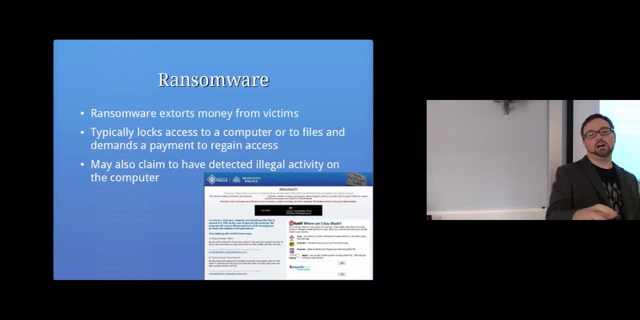 to have detected that you've done something illegal. so it'll say: I've detected that you've been accessing this, this and this and therefore, if you don't pay up, the police will be after you, essentially. and then wasn't there a story recently where someone actually committed suicide after receiving one of 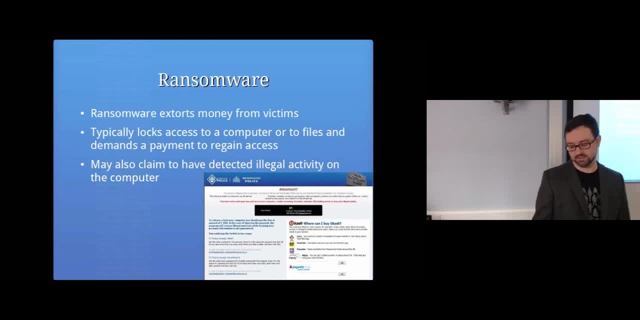 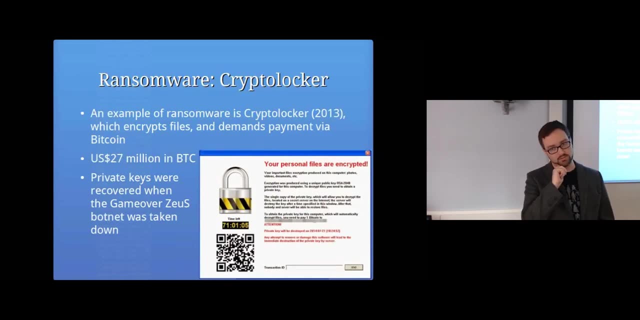 these threats. so, yeah, it's, you can have pretty serious consequences. you can have pretty serious consequences, but the probably the most likely one that you would have heard of is crypto locker- so that's just recently, last year- where it encrypts all the files on your computer, so that it's it's basically impossible to get the original files. 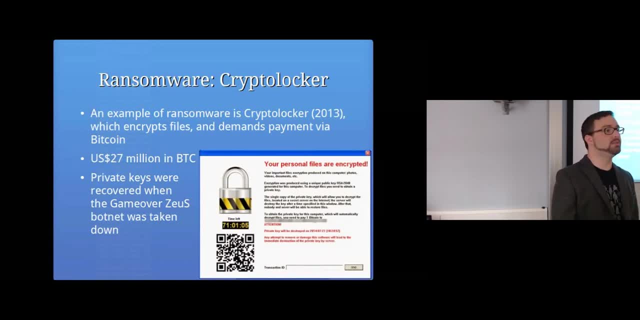 back unless you pay up, and the payment in most cases was by Bitcoin and, looking at Bitcoin transactions, we can see that something like 27 million dollars was actually paid by people that got infected- and there were. essentially, it was impossible to decrypt because the actual the encryption was done with a private key, which was never 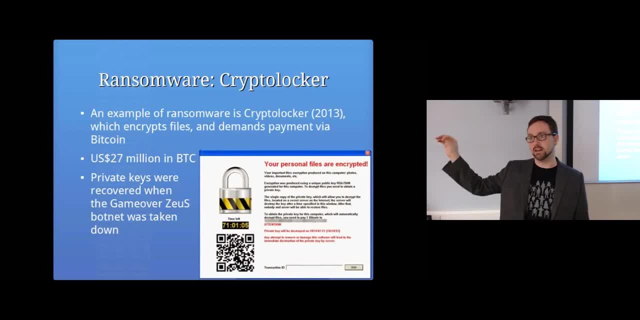 on the computer. to start with, the public key of the attack of the attacker is used to encrypt all of your files, and then the only way that you could decrypt it is if you manage to get access to that private key and obviously the attackers, anyone that has that. so if you want it, you have to pay up and the the official. 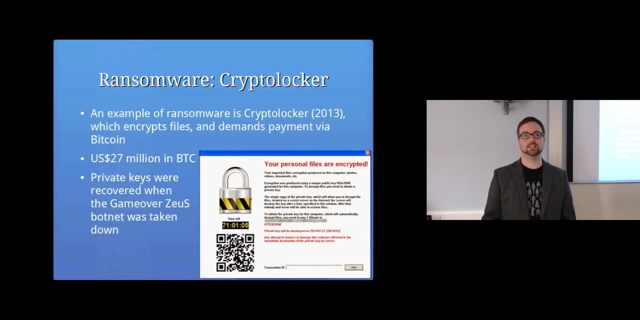 advice is obviously: don't pay up because you're paying. basically it gives gives them more incentive to try harder to do this more to other people. but when it's your files that are that are being held ransom, then I guess you know your decision-making process might also involve. you know what it is that you've. 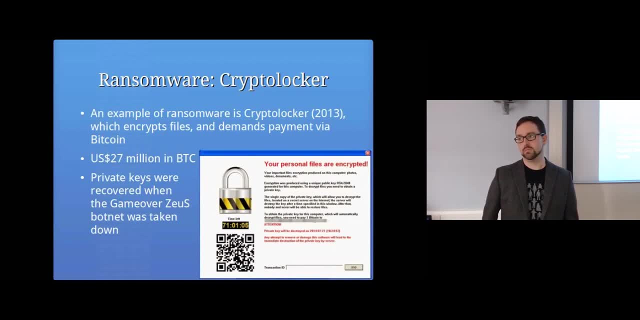 just lost. they did, they did unlock it. if you paid up, so yeah, well, I guess, I guess if people knew that they weren't paying, they weren't giving them access to their files, then people would actually not be less likely to pay. but also, if you use 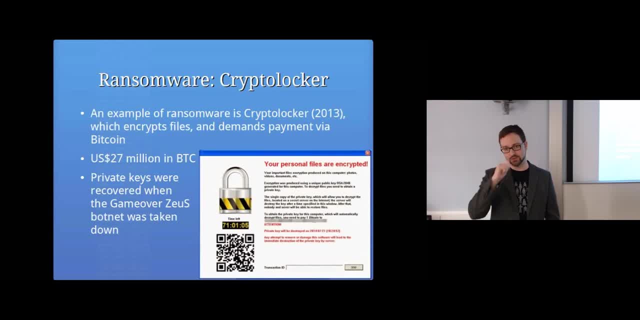 antivirus offer to get rid of the crypt crypto locker from your computer, then the head. you also had no way of getting files back unless you've reinfected your own computer so that you could decrypt the stuff. so yeah, there was a a very big takedown of the botnet, which is the game over Zeus botnet, when 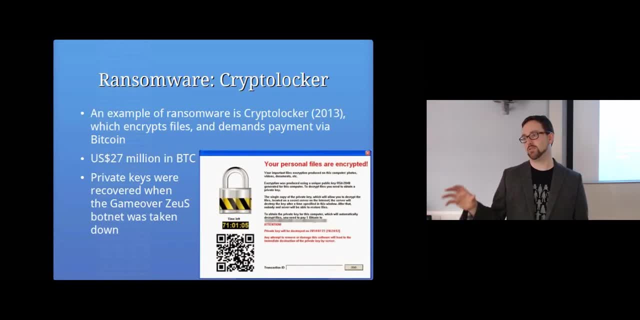 that was taken down, they did recover private keys for from a bunch of people that had been infected. so it is, if you're lucky enough to be one of those people whose private keys was part of that, then it might be possible. you know, if you're lucky enough to be one of those people whose private keys was part of that, then it might be possible. 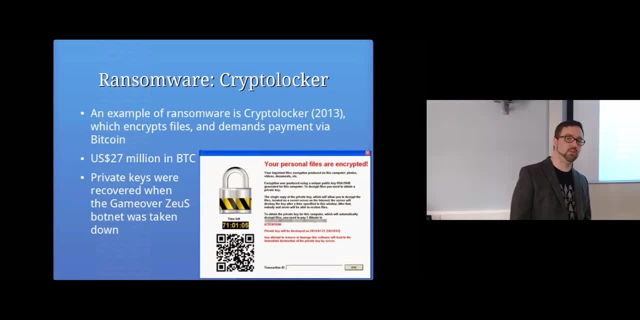 to decrypt your files now, and I believe there were some versions of this software that had us, like a programming mistake, which also allowed you to recover your files. but in most cases, if done correctly, it's just impossible to get your files back without their, without the attackers. help on that note. 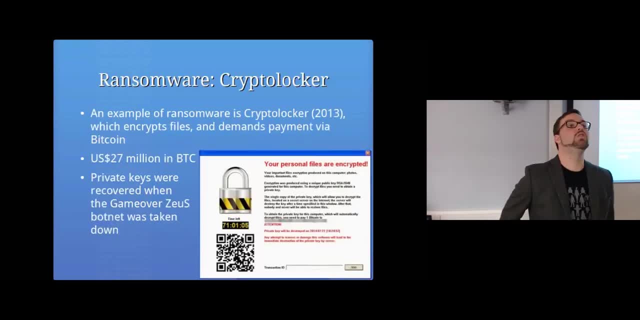 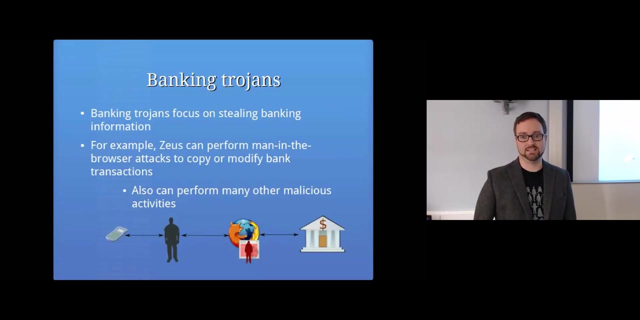 banking Trojans, actually, no, sorry. so who here knows someone who has actually been hit by a crypto locker? do you know? does anyone here know someone who's actually been affected by crypto locker and show of hands? okay, a few, a few. did they pay up? they pay up? no, no, so so in that case, so banking Trojans are Trojan. 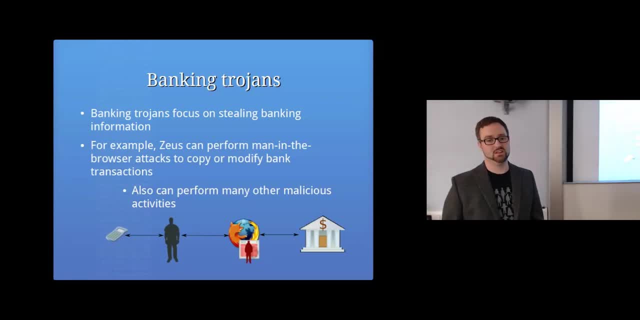 horses that focus on stealing banking information. so Zeus is probably one of the most famous or most popular recently and it can perform man-in-the-browser attacks. so, essentially, what a man-in-the-browser attack is? where your actual computer is infected to the point where it changes what your browser is doing. so when you 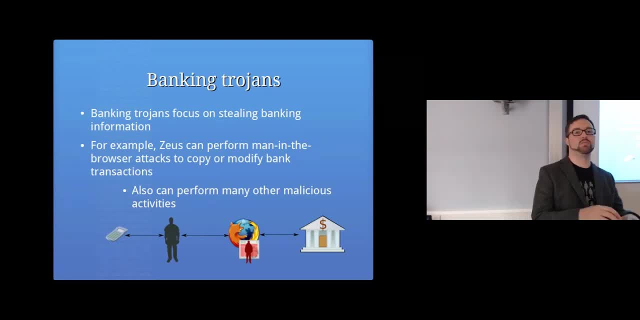 log into your bank account, you, you log into your web browser and you basically tell your browser: transfer some money to this person. the browser then talks to the web server in an encrypted, you know, using SSL encryption and everything like that. so it shouldn't be possible to do a man-in-the-middle attack, but if you can, 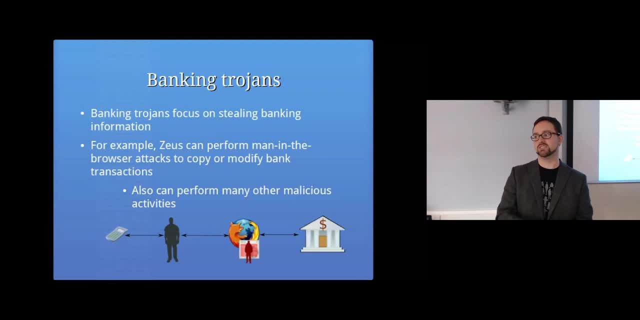 change what the web browser is saying. you can still get into that transaction and change the message that's been sent to the bank. so you can say to the bank: actually make that $2,000 you're sending and actually make it to this person. and if you have like an authentication token, then you know if they're controlling. 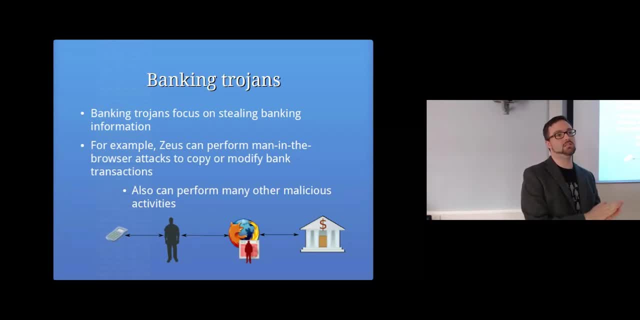 what's coming out of the, depending on what you need to type into that you. they might trick you into typing what you need to into that authentication token, and I mean I wrote a man-in-the-browser attack that did just that. obviously I never released it, but so it's not that difficult, it's you just. 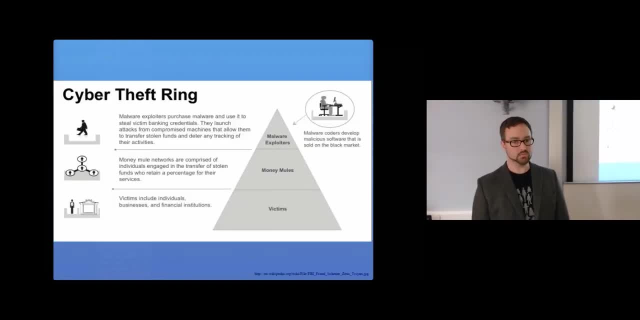 you can just write it as a Firefox extension. so just an example of how some of these like things can work is you can have a. basically you've got the person who writes the, the malware. they sell a copy of that malware on to someone on the black market. a malware exploiter purchase the malware and they they. 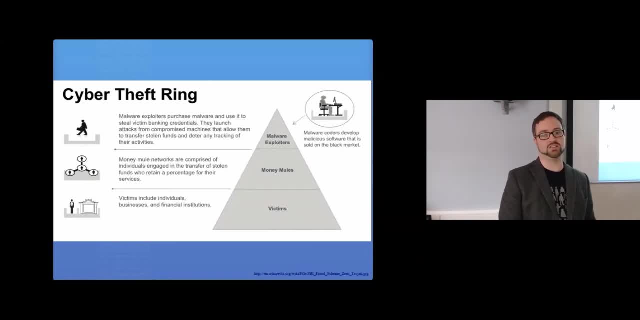 basically use it to steal banking credentials and information and then they can then access those compromised machines to transfer the funds to somewhere else and then basically they would send it to a money mule network. so a bunch of people that work together to basically transfer that stolen money and work as a middleman and they get paid a. 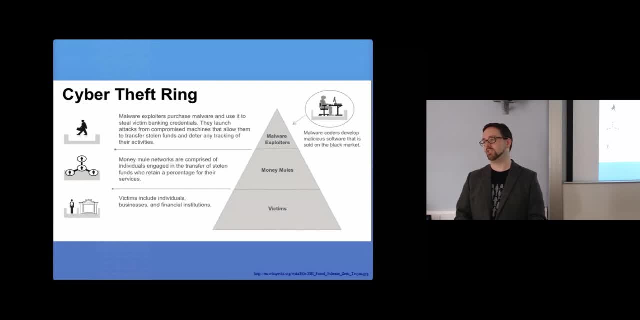 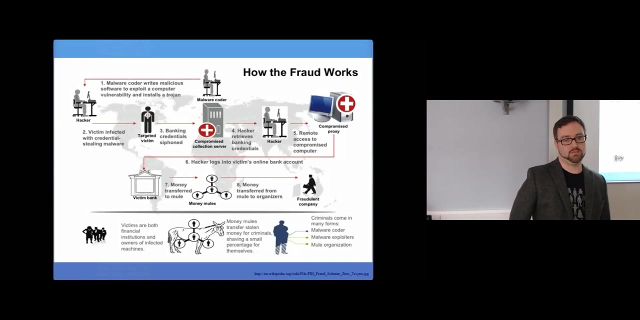 percentage for being like in the crossfire, basically, but it gives the, the malware exploiter, a buffer between the police and them, and the victims are just people that you know- individuals and businesses and financial institutions. so it kind of works a bit like this. so I think I 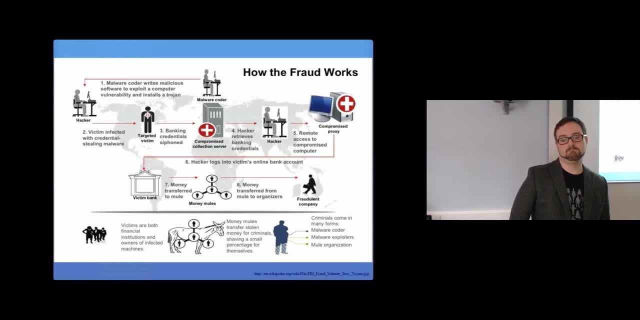 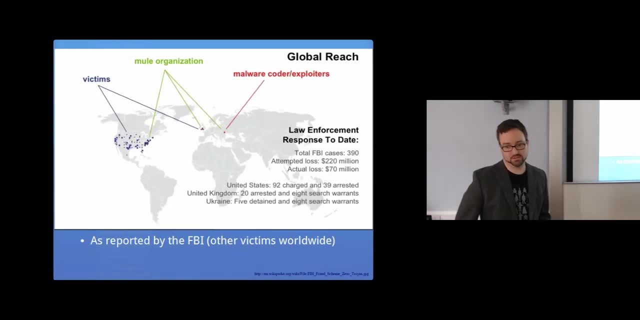 essentially just described it. so yeah, and it's everywhere. and obviously this picture comes from the FBI, so it's all about the fact that they're American victims, but the actual people who wrote the code and the people that are transferring money are not necessarily within the same country. so as soon as 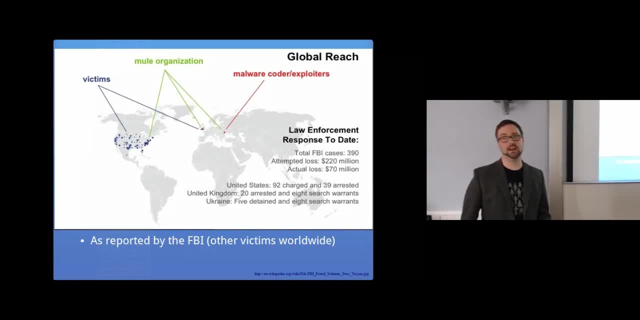 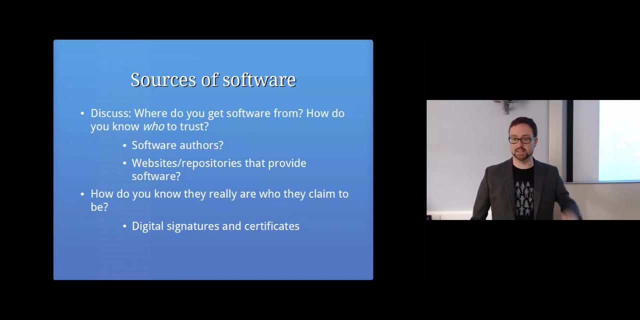 you have multiple jurisdictions involved, it also becomes very hard to actually go after people legally, because if you, if you have people across jurisdictions, the legality becomes difficult to follow through with, but not impossible, depending on the level of you know what has what's happened. so, sources of software: where do you get your? 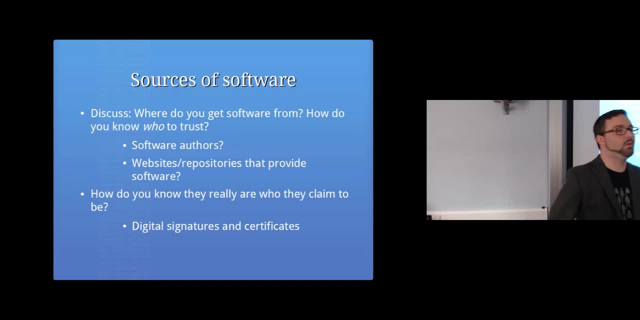 software from guys like: how do you know, how do you make a decision about what you should install on your computer? maybe just could someone just suggest where they get software from. yeah, okay, so if you're torrenting software, how do you know that you can? how do you know that you can trust the software? 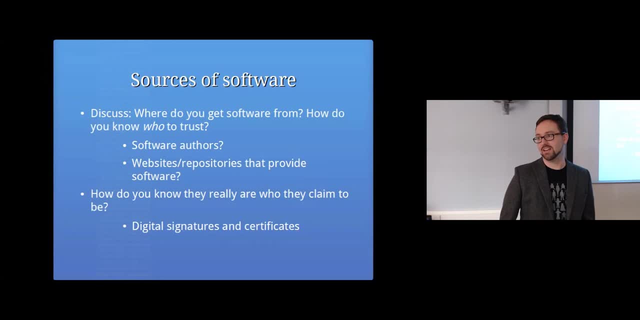 peer review. peer review. and what reading comments from other people that have used the software, and do you think that they someone would know if they had a keylogger installed on their computer? how many comments are you are we relying on and how educated are these people? 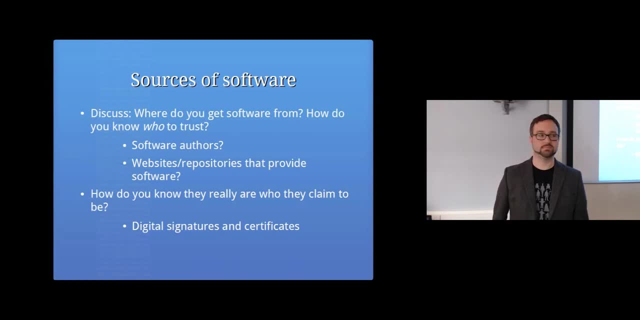 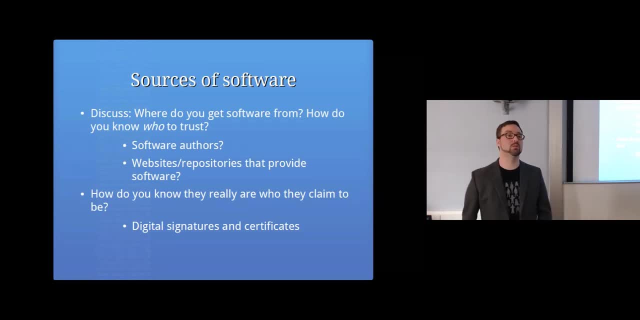 yeah, probably not the most reliable source. I'll talk about ways you can protect yourself against software that you might not trust in a minute. so it's not that you can't run this software, but I've definitely wouldn't just install it on your main Windows system because you'll be doomed probably, maybe, possibly. 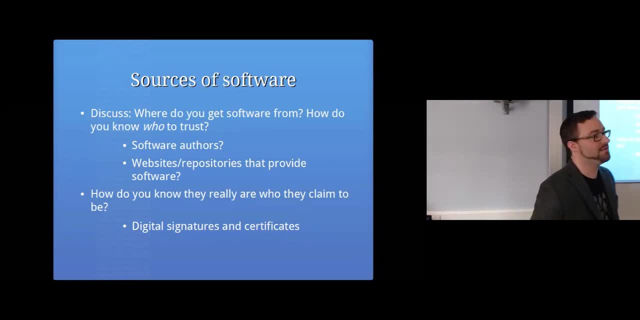 any other ideas where you might get website software from that? you may or may not trust company's website. so, for example, if you wanted a copy of a, the data set that you don't have, you could probably go to a site that that might be be there and, like Google, for you can access it, so you can see it. how do you? 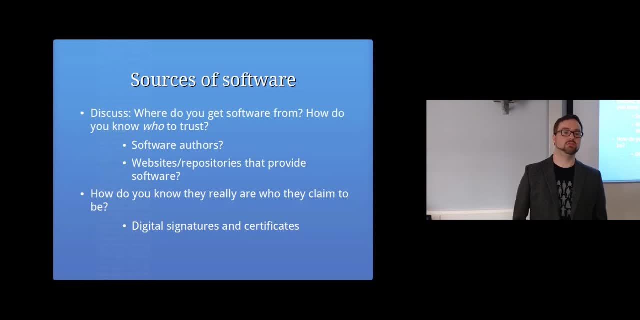 what's the? how do you want to use it? if it's just like as far as downloading it from a baby, do you download it right? so you do. how do you get to AVG website, whether it's my video, or can you give me an example of a URL that you might type? 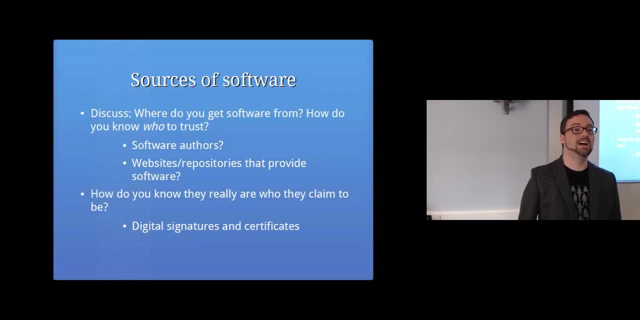 in wwwAvgcom may or may not be their website, but also, if you didn't type HTTPS at the beginning of that website, you're not using encryption, you're not using any verification that the website you're connecting to is actually their website, So you could be a victim of a man-in-the-middle attack. and actually connecting to someone, 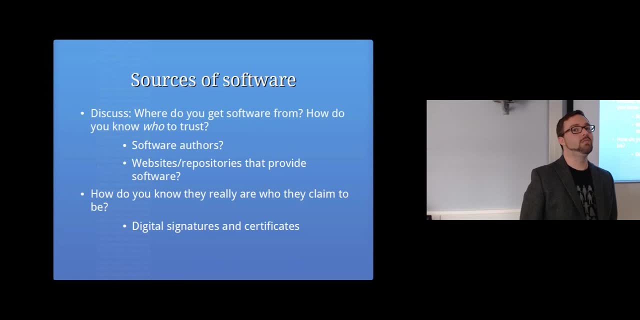 else's computer, the attacker's computer, for example. How else might you go? Basically, you're doomed, is what I'm trying to say. So yeah, you can do these things. There are ways. It's all a matter of it's a scale of likelihood, right? 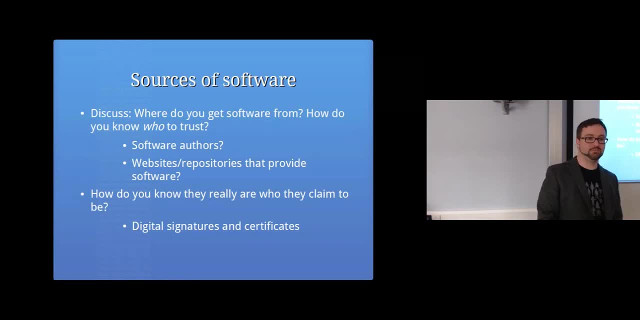 If you go to their website and there's no certificate there, you're not using a secure connection. that's more secure than getting it from a torrent, But there's still some risk there. So one of the ways that you can kind of be sure that they are who they claim they are. 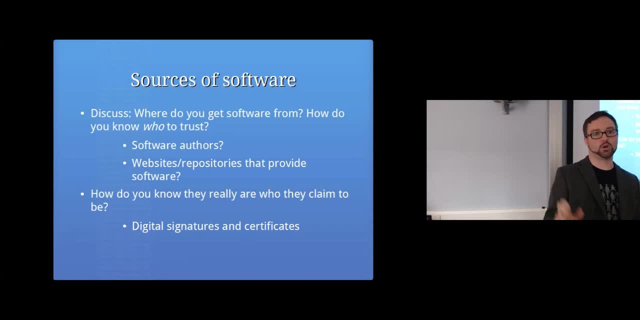 is to look at digital signatures, So a digital signature can prove the author of the software. So on Windows, when you run something it'll say: do you trust Microsoft Corporation? You know to run their software or whatever. And in that case if you are confident that you trust Microsoft, I mean you already do. 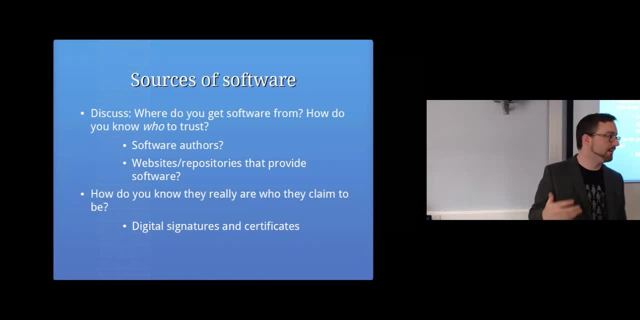 if you're running Windows, So then you might agree to run that software. But if it says: do you trust unknown author to have the software, then you might reconsider: where did I get this software from? how much do I trust it? So what I'm going to do is I'm going to go to Microsoft. 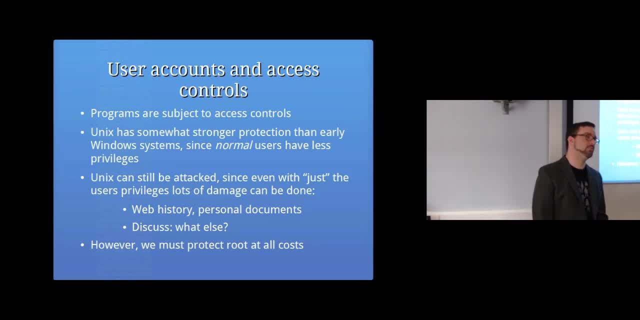 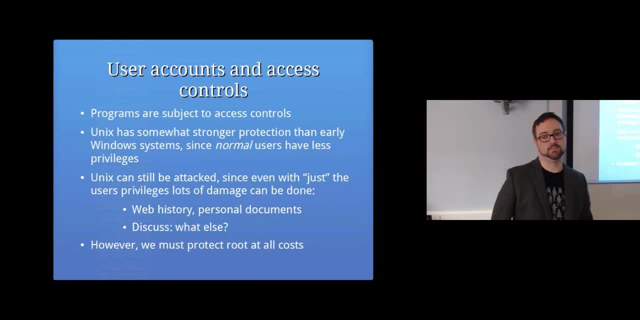 programs can access what or what people can do what on what computer, And normal users have less privileges. Back in the day Unix had normal users and super users. long time Windows only had administrators. so if you used anything before Windows XP, then everyone, when you're logged in, was just running with. 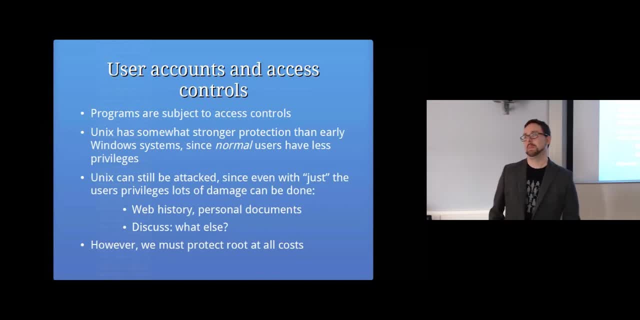 full access to everything on the computer. Windows XP had system administrator accounts and normal administrator accounts, but you basically nothing works if you don't, if you're not an administrator, because all the software wasn't designed for that feature, but it was a step forward in terms of security. but if you're using Windows XP, you kind of have to log in as 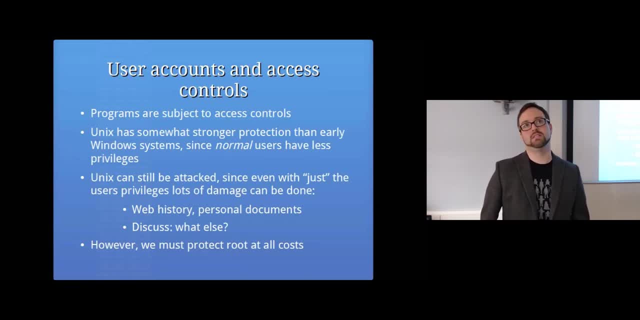 administrator if you want stuff to work, but then from then on stuff has him. it has improved where you can be logged into a computer and not necessarily every piece of software you run will be able to do anything on your computer. so the moral of the story is: don't log in as administrator on your home computers. 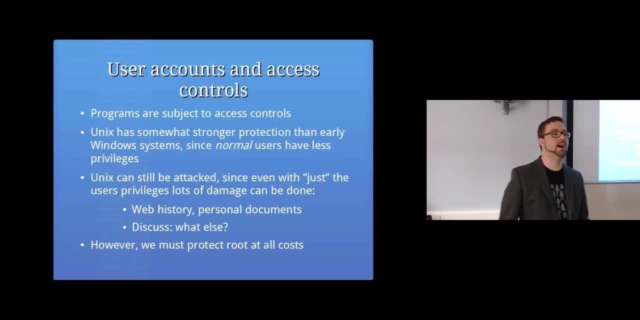 unless you really need to, because as soon as you do that, then if you accidentally run a piece of software that you don't trust, then a lot worse stuff can happen than if then if you just logged in as yourself, um, and if sometimes you can actually install software without being an. 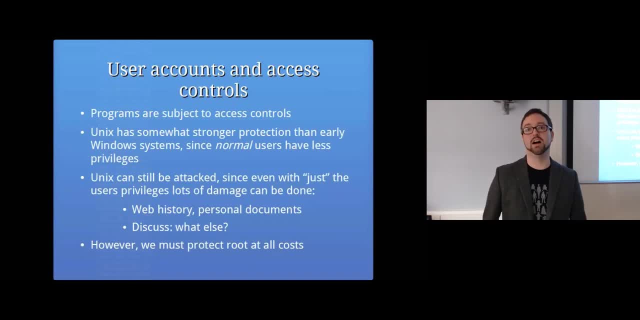 administrator, and that's probably the safest way you can do it: you just create a new user account, install some software onto that without you know, without actually elevating to administrator, but then obviously, but there's still a lot you can do. if you, if a piece of malware just runs as a normal user, it still has. 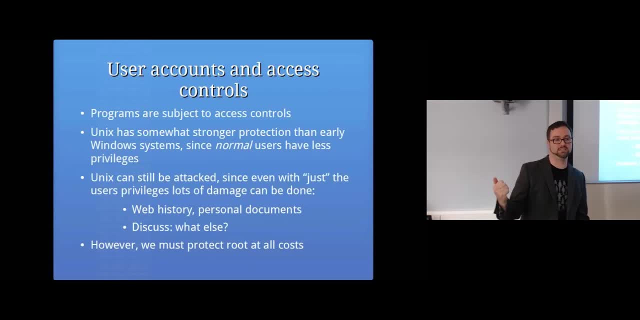 access to a bunch of stuff, right, so still got access to all of your web history. it still has access to all of your personal documents. it still has the ability to attack- you know you- using your banking website. but what it can't do is actually change your operating system. but we 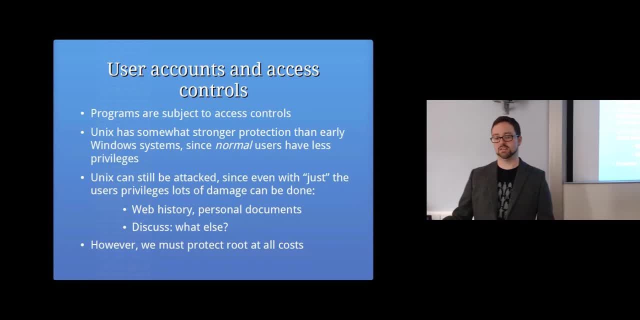 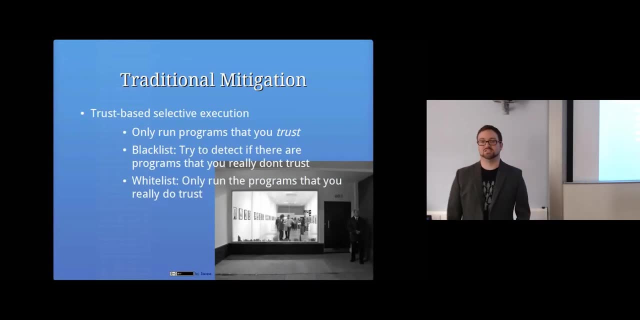 really do need to protect root at all costs, the administrator access. so how can you do that? so the traditional way of protecting yourself is: just don't run stuff that you don't trust. so trust based selective execution. so I'm only going to run certain programs. and how do? 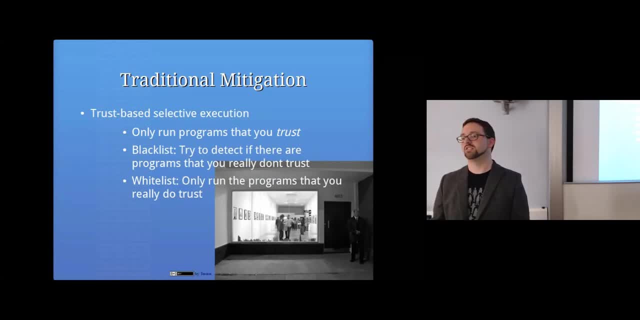 you decide that, well, you might have a blacklist of programs that you don't trust. for example, you have anti-malware that has a list of programs that it doesn't think you should run, so it'll stop you before you even start to run it. or an even more secure way, but practically impossible, is to include 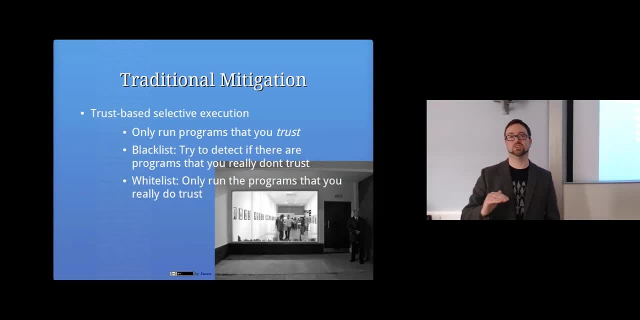 have a whitelist. so I'll say I'm only going to trust these programs, or all programs from these places, and if you have a real lockdown corporate network, it might be worth doing that, although a few years ago one of the companies that provides that service got hacked, so but but you can actually, you know, use a. 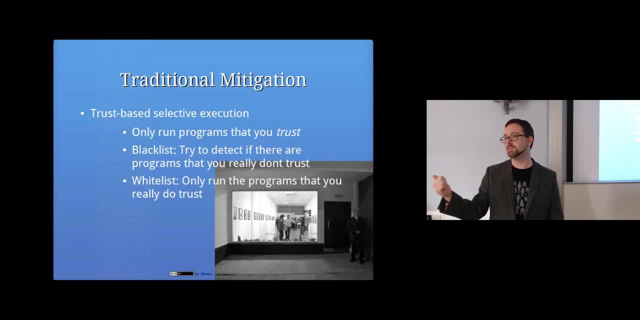 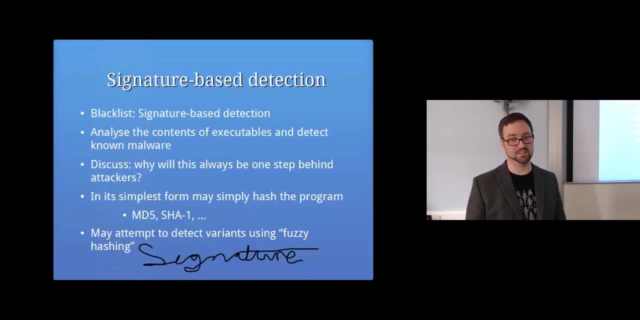 whitelist within your company and say, okay, I'm only going to run Adobe software and Microsoft software, for example, and that would make your computer very secure but very hard to use if you wanted to do anything else. signature based detection is basically when you base those blacklists. 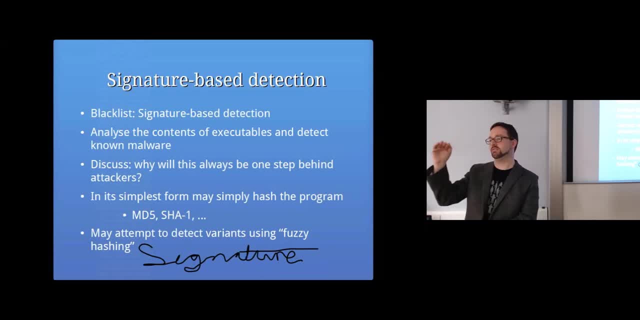 on a blacklist and then you have a blacklist, and then you have a blacklist or whitelist off, looking at the contents of a file and trying to detect whether it looks like something that's been seen before. yeah, zone alarm sort of firewall, right. so that's that's like after you've already trusted the program. 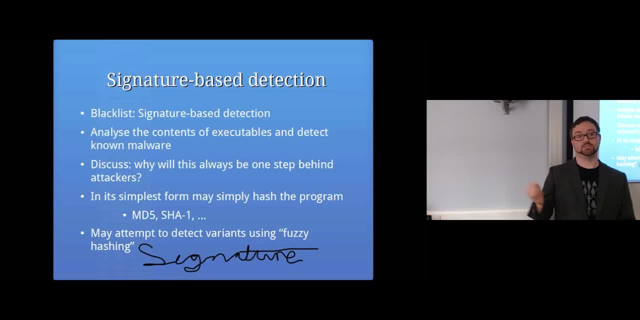 to run what it's allowed to do in terms of network traffic. I guess what I'm talking about now is: how do you decide which programs you allow to run in the first place? so, like a lot of antivirus software will be based on a signature, it might- I mean a lot of. 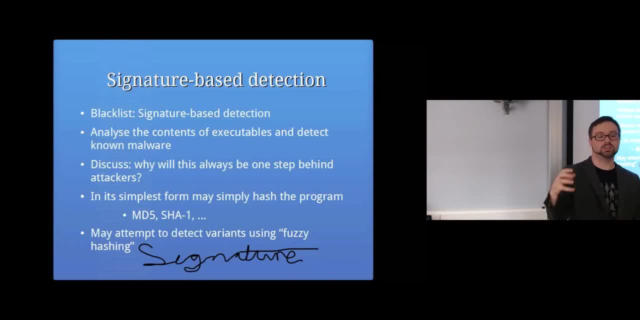 firewalls and IDS's and things are signature based as well. but in terms of deciding which programs to run, we look at the contents of the of the program and say, oh, this looks like a virus I've seen before and it might be slightly different, but are not similar enough that it matches the signature and but 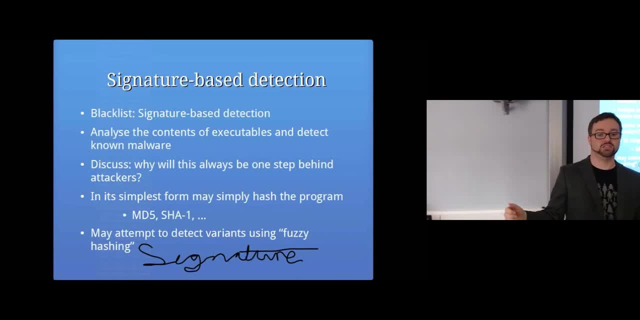 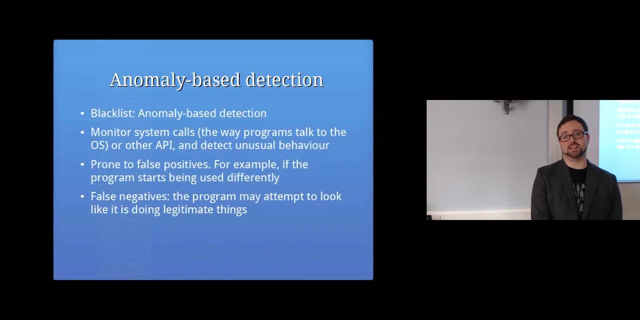 the simplest kind of signature might just be like a one-way hash function like md5 or sha, sha1 or whatever. but then as you just change it slightly, then it wouldn't match that anymore. so you've got kind of fuzzy hashing where you can detect programs that are similar. anomaly based detection is where you detect the. 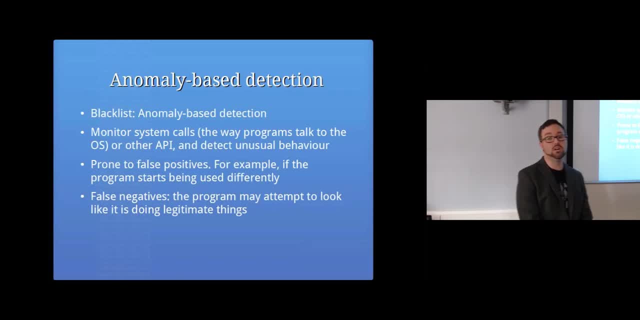 software is doing something and probably shouldn't, or that it's never done before. so you might look at the way that the program is talking to the operating system, where you might look at the files it's accessing. but the problem with using anomaly based detection is that it's prone to false. 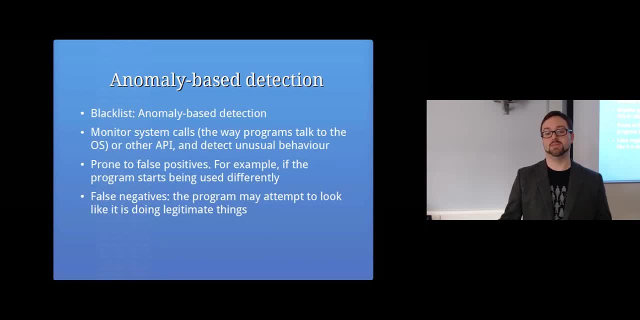 positives. so if you have a perfectly fine piece of software but you start using it differently, it might trigger an alarm. well, this programs have been used to access that resource before and it's like, well, I've just never used it this way before, but it's just I'm still using it- or a false negative where it actually. 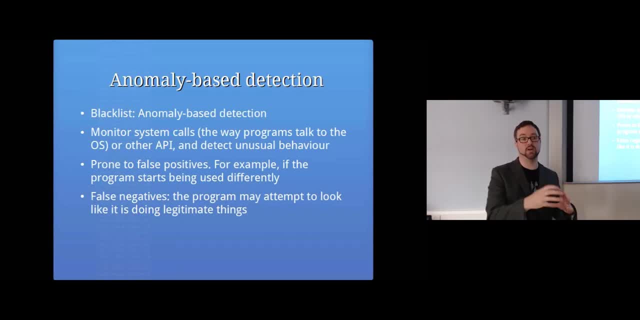 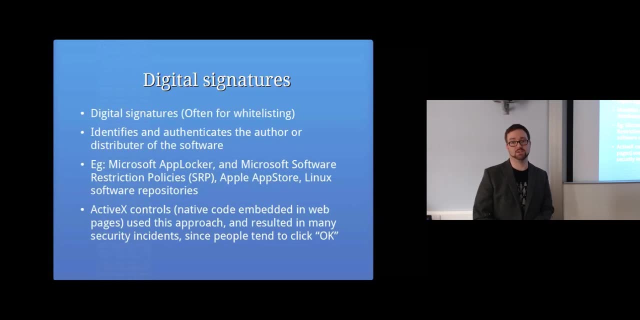 actively tries to make it look like it's doing something similar, but it's doing something bad, so it can often fool those kinds of detection. so I said before, digital signatures can be used for whitelisting and you can basically identify and authenticate the author of the person who's distributed the software. so, for example, you can use 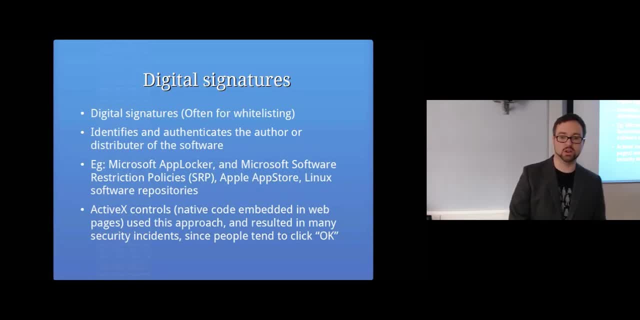 Microsoft AppLocker or Microsoft software restriction policies or Apple App Store or Linux software repositories are all based on that, where you can basically have signatures attached to certain executables and you can say which of these you trust and which ones you don't. ActiveX controls because it was a horrible idea, but basically one of the first ways that. 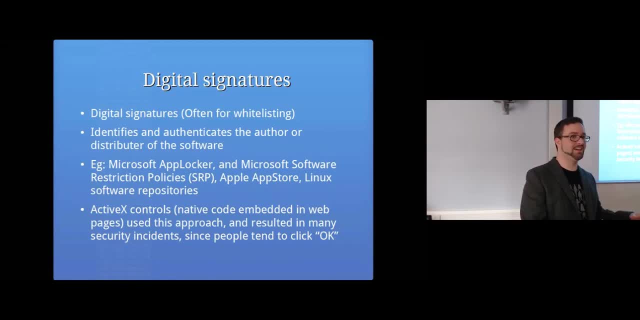 websites provided like cool features was to use ActiveX. but as soon as you could browse to the website, it pops up and say: do you trust this person? and you click yes, and then they're running a program in your computer. I have very bad in hindsight, a bad idea, but at the time I'm sure it made sense. so I'm just going to leave it at that for now. 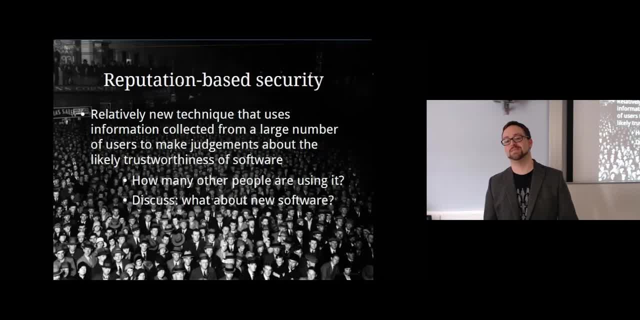 sense to someone. reputation based security is basically where you look at information collected from lots of people and like, if this virus has been seen, like this piece of software is used by thousands, of thousands of people and no one's complained about it, then it's, we will trust it kind of thing, and so for. 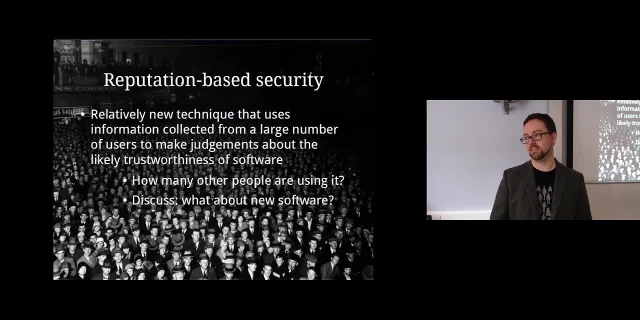 example, like the new Norton and McAfee and things like that. they often use these cloud-based, you know things where everyone sends information about everything they're accessing to them and then they can use that to decide whether it looks suspicious or not, but it kind of. it also depends on. 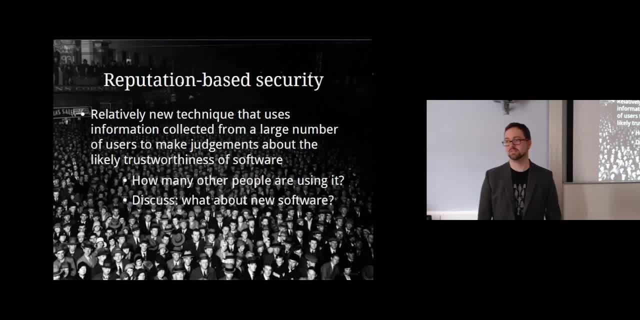 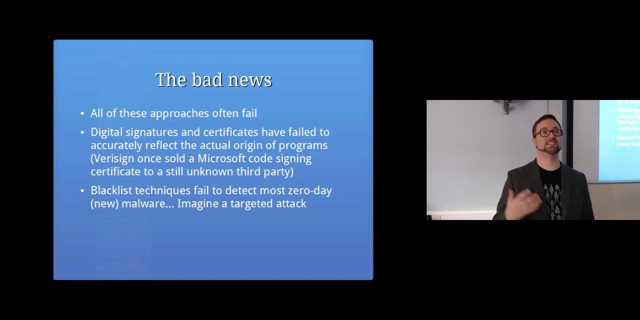 how many people are using the software, and there might be niche pieces of software which are perfectly fine but not used by many people. and obviously new software. you know it's not going to work. so bad news is: all of the approaches fail, like everything that we have to protect ourselves against. 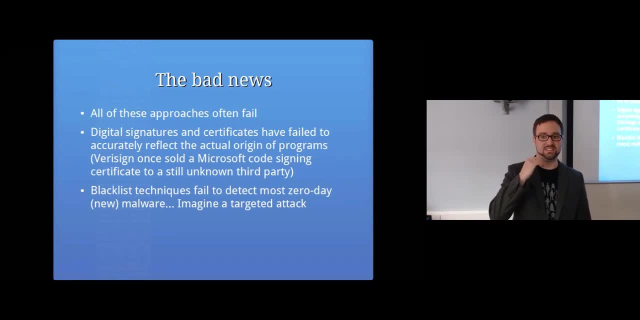 malware. they often fail. so digital signatures and certificates have failed loads of times. so once VeriSign actually sold a Microsoft code signing certificate to someone on the internet. so they said: I'm Microsoft, can I have a certificate please? so there's someone out on the internet that had the ability to just sign stuff, so it looks. 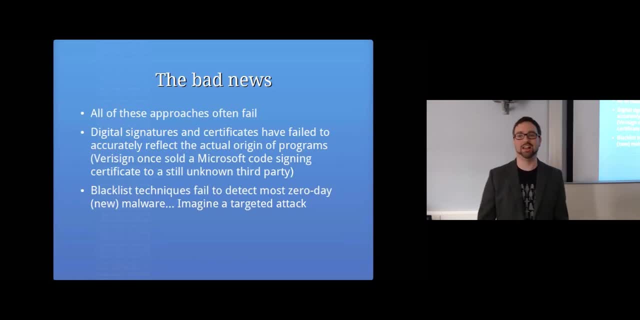 like it came from Microsoft. that's a major problem, the whole idea of being able to use certificates to trust people. it only works if the people that are verifying who gets the access to certificates are actually doing their job. but also, blacklisting techniques just fail to detect, almost like. 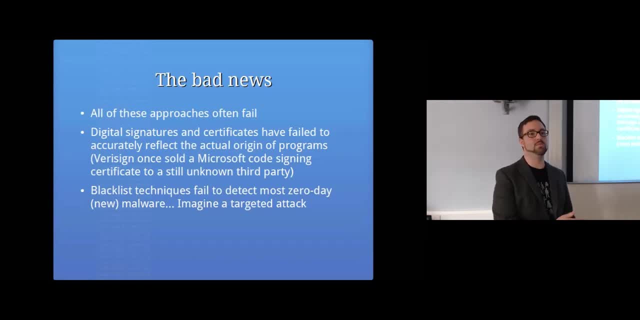 things that are not being used by the people who are actually using the, everything that's new. so as soon as you- if you, if I- go back to my office and write a new piece of malware and send it to- it's very unlikely- your antivirus software it's going to detect that it's that it's a problem because it's never. 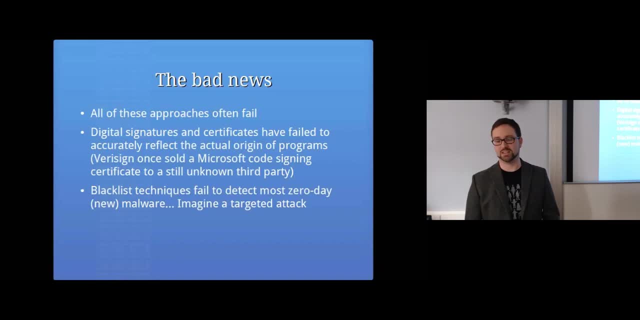 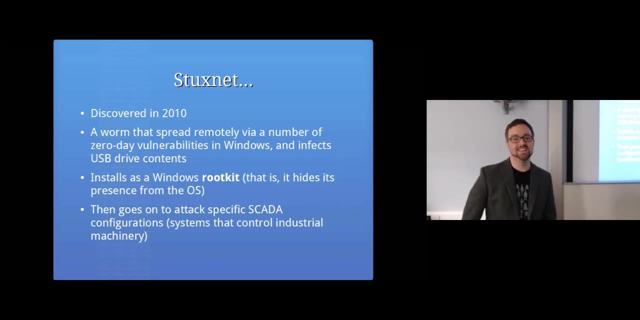 seen it before, so you know. obviously it doesn't protect very well against targeted attacks. and Stuxnet obviously is a big one discovered in 2010, basically spreads between Windows computers and infects USB Drive contents and installs as a rootkit. then it goes on to attack specific SCADA configurations. so and 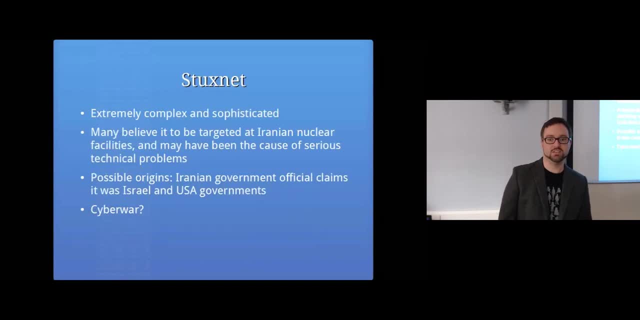 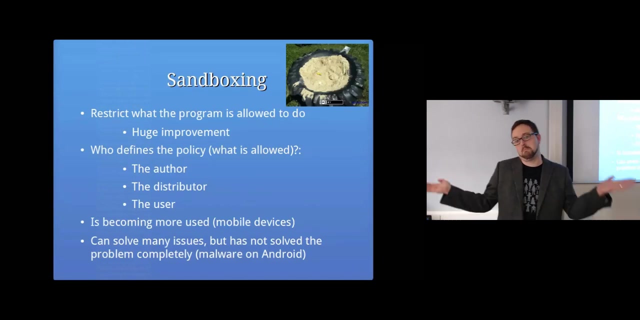 that's the software that uses controls industrial machinery. so it's incredibly sophisticated piece of malware and many believe- pretty much everyone agrees now- that it was actually targeted at Iran's nuclear facilities and allegedly created by Israel and the US government. so cyberware, cyber warfare, maybe sandboxing- so one thing that you can do just to protect yourself is to use a. 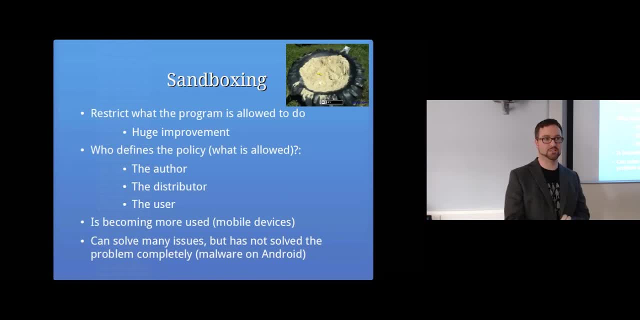 sandbox. so if you've got your torrented software- which I'm sure is perfectly legitimate and you want to run it and be sure that you're safe to do so, then you can use a sandbox so actually can find that program so that when you run it it 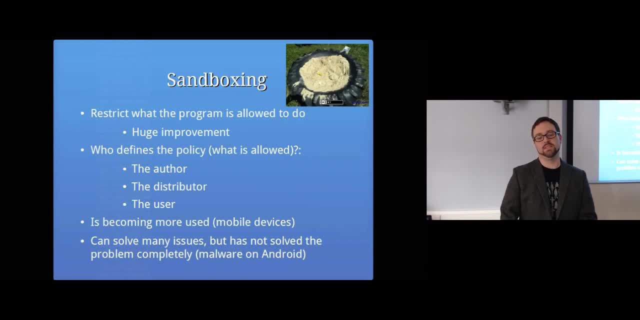 can't go off and damage your computer, so you can, and there's a few different ways of doing sandboxing, but it doesn't stop you from doing it if you want to do it and solve the the problem completely. so, for example, we've still got malware and 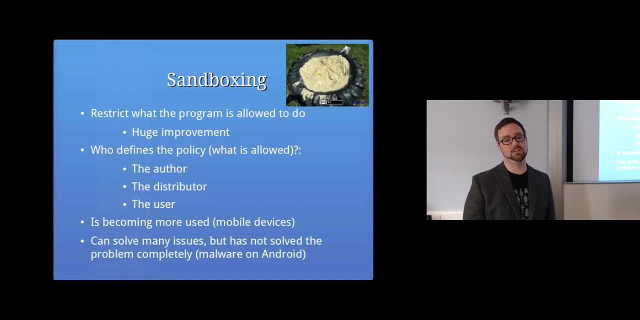 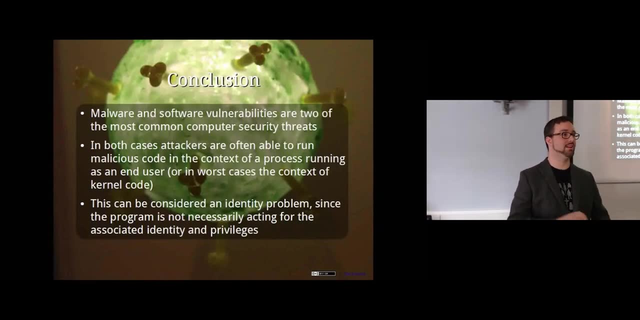 Android and it uses a sandbox. but you know there are a few different things you can use to protect yourself if you're using Windows. I do actually recommend sandboxy is quite a nice way of just running a program and it can't write to the registry or to files. it has its own kind of space that it sits in. so 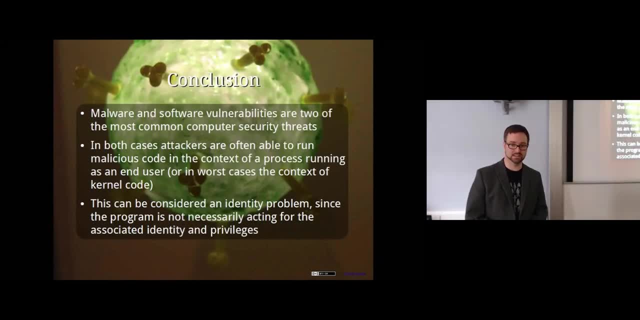 in conclusion, and so malware and software vulnerabilities are very common security threats. in both cases, it allows and attacker to run malicious code in the context of a process running as the end user or, in worst case, as as the kernel. and it's essentially an identity problem, because we're forced to trust that the program is acting on our behalf when it.